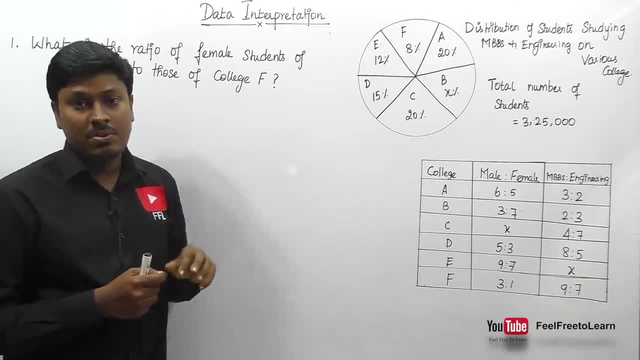 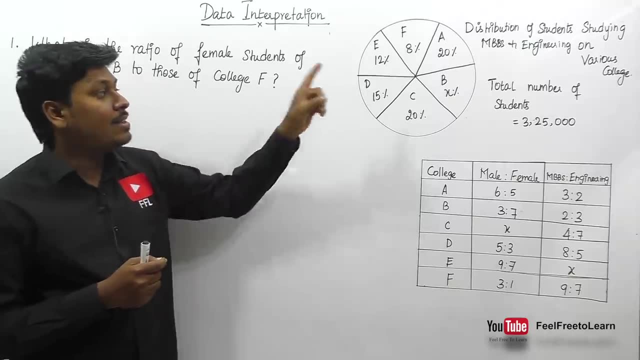 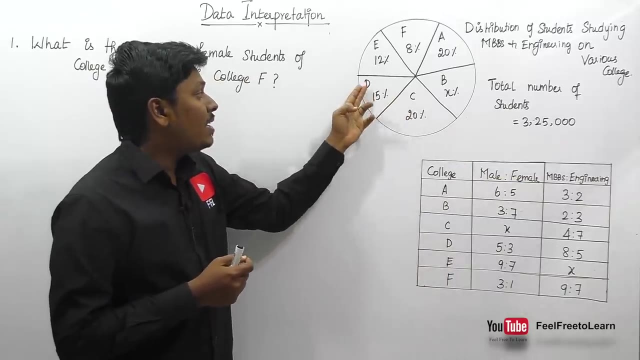 students are studying. So, out of this, 3,25,000 students, all the students are studying in a different colleges, that is A to F, and they are studying two fields. One is engineering and second is MBBS. So, out of this, 3,25,000 students, the college C has 20 percentage and college D is 15. 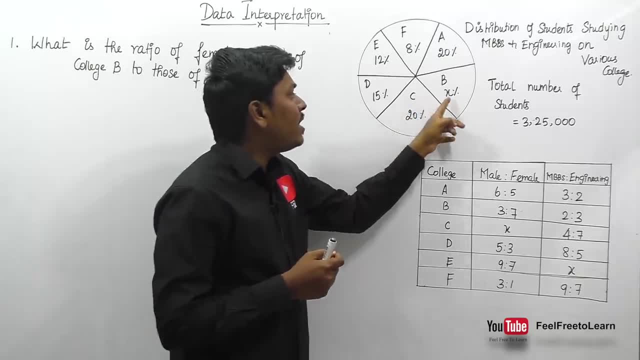 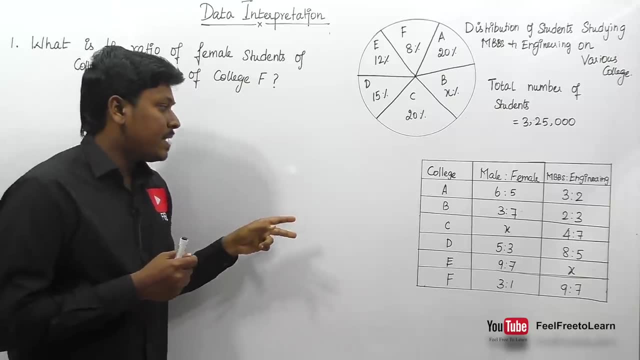 percentage. college E is 12 percentage, but they didn't give the value of B right. So college B, that is X percentage. So we need to find what is the value of that, Okay? secondly, they have given a table chart and here the table chart that is from college A to F, male is to female ratio and. 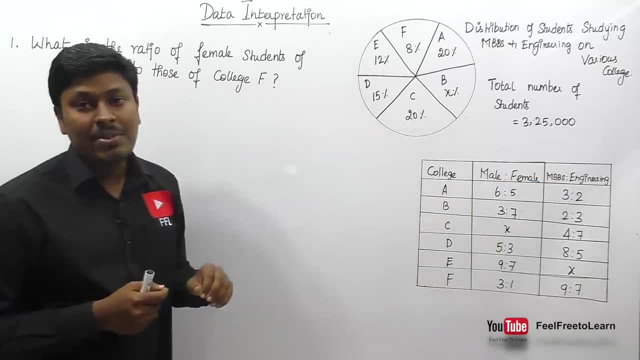 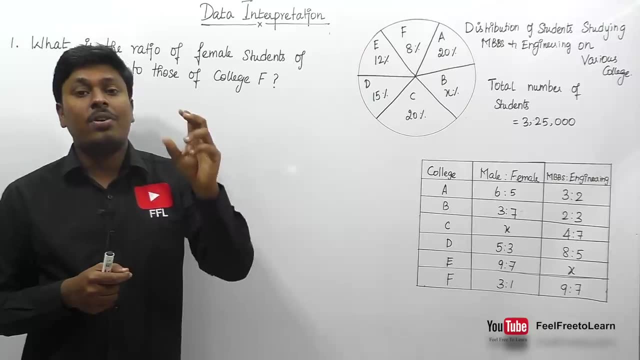 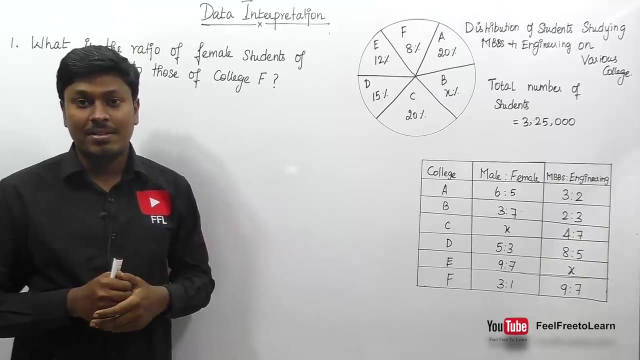 the students who are studying MBBS and engineering. that to all the values are given in a ratio. So, friends, the table chart is completely for MBBS and engineering students ratio and for male and female ratio in all the colleges and the pie chart that is total number of students who are distributed into various colleges and some 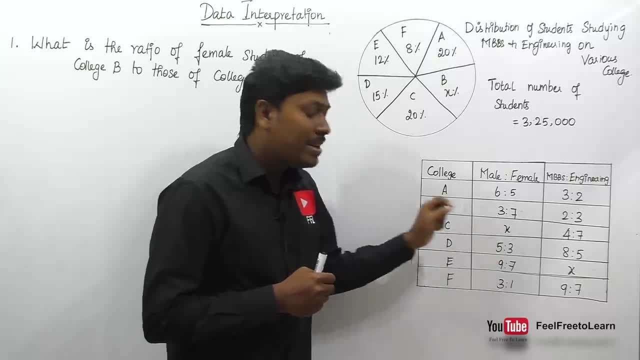 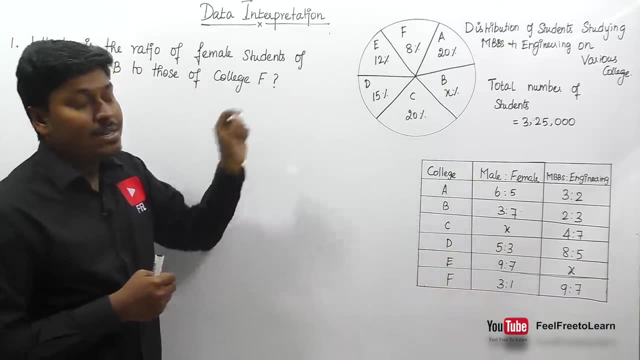 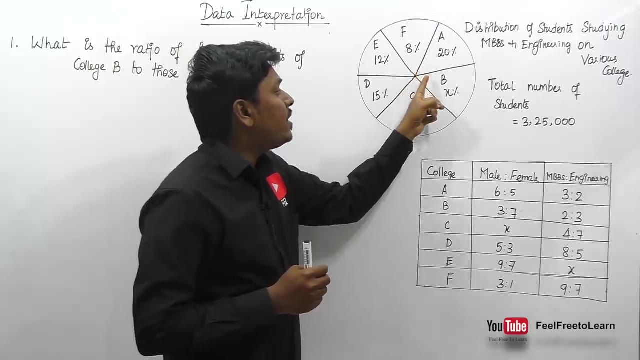 of the values are not given. in the table chart, that is C, male is to female ratio is not given and college E, where MBBS and engineering ratio is not given, but here in the pie chart that is B is X percentage. So, friends, before solving this, always remember that this pie chart, we know that this complete. 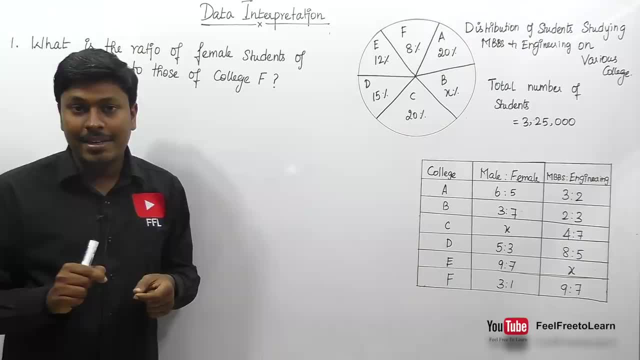 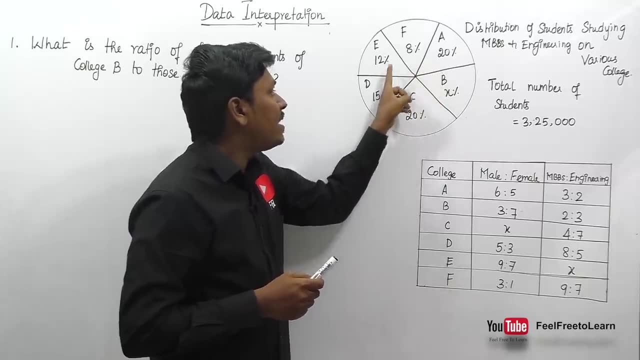 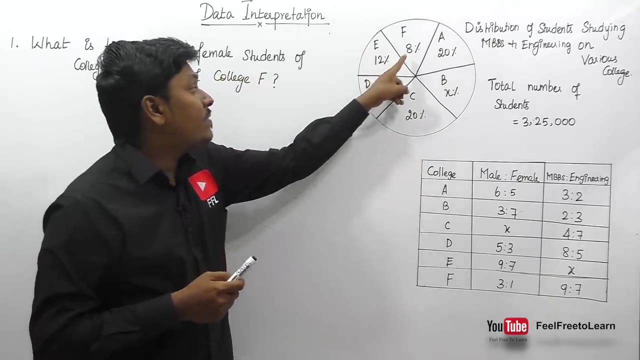 angle is 360 degree. If it is a pie chart, 360 degree- always 360 degree- is equals to 100 percentage. If I count all the values, it should be definitely 100 percentage, right? So, friends, 20 plus 20 will be 40.. So 40 plus 15 will be 55.. 55 plus 8- I think this- this will be 20, right. So 55 plus 20 will be. 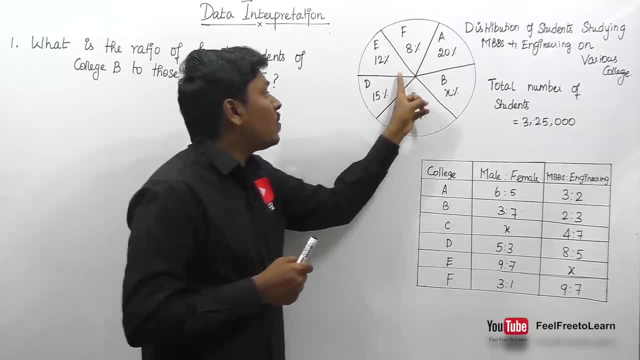 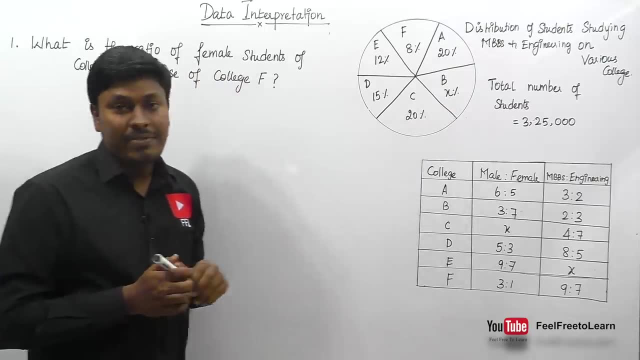 75. So the total is 75. We know that this total circle should be 100 percentage. So 100 percentage minus 75 percentage, the resultant B will be 25 percentage. So I can say that the value of B, that is X percentage, will. 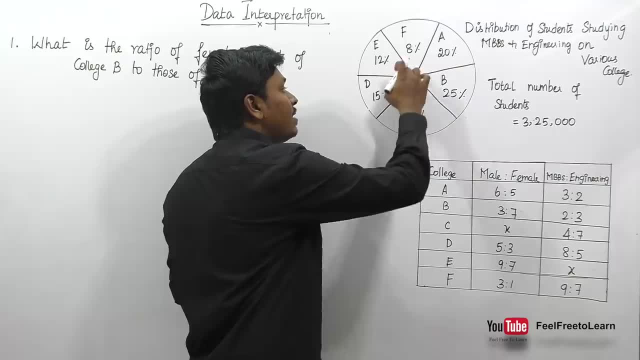 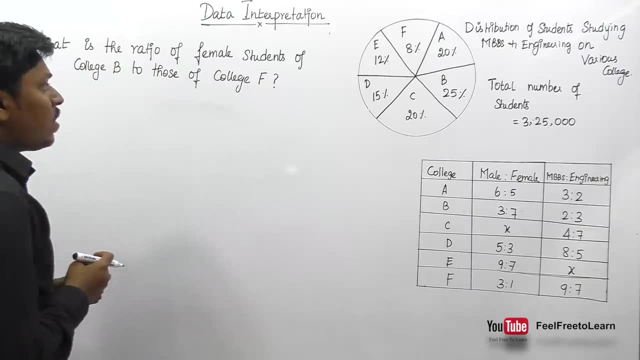 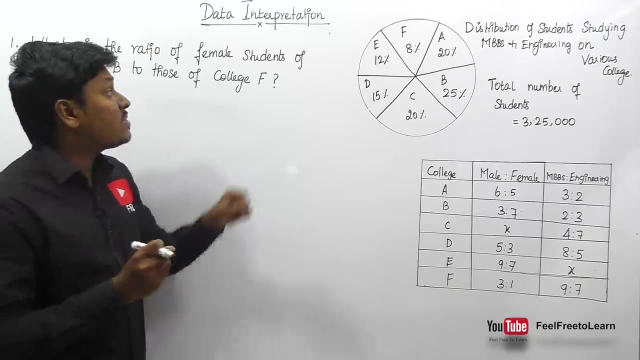 be 25 percentage. So, friends, always remember that this total circle should be 100 percentage. Okay, friends, let me move on to the first equation. What is the ratio of female students of college B to those of college F? So, friends, our target to find the ratio right, that is for the 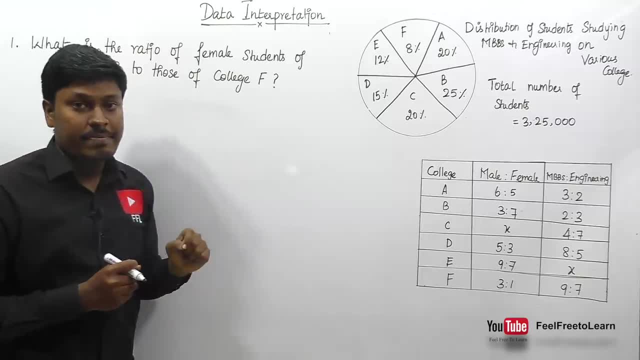 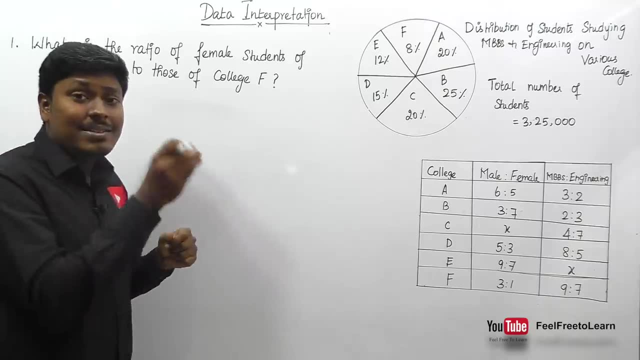 female students of college B to those of college F. We need to find the ratio that is for female and college B to the female that is in college F. Friends, they are not particularly asking whether it is an MBBS or engineering right, They are just targeting the total number of. 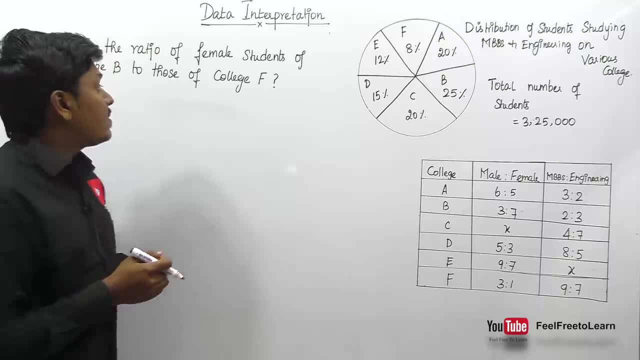 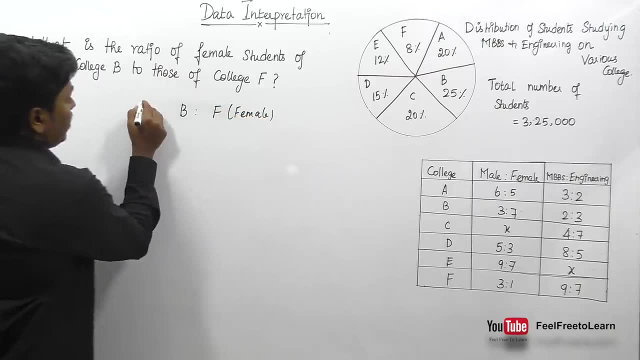 students in college B, that is, female students. So, friends, our target to find the ratio, that is B to college F, only females. right, Okay, The two. you have two females right to college B, female to college F, female. So, friends, listen carefully. First of all, let me target. what is college B? College B, the total number of students is 3,25,000. 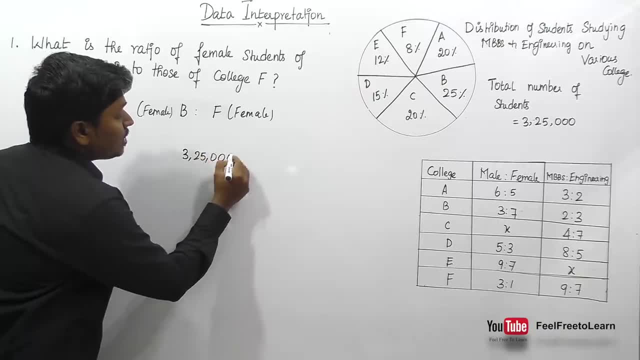 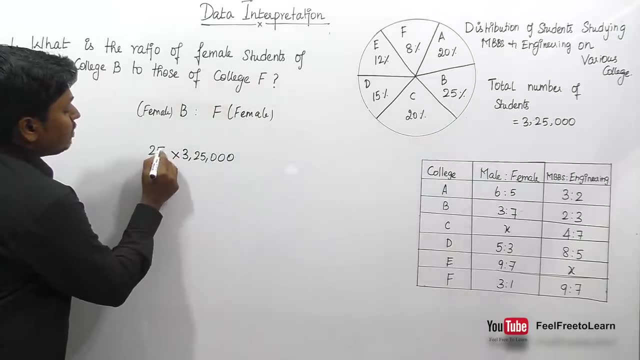 So, out of this, 3,25,000 students, how many students are studying in college B? friends, 25 percentage of students are studying in college B. So I can say that 25 percentage of students are studying in college B. So, out of this, 25 students, our target to find only female in college B. 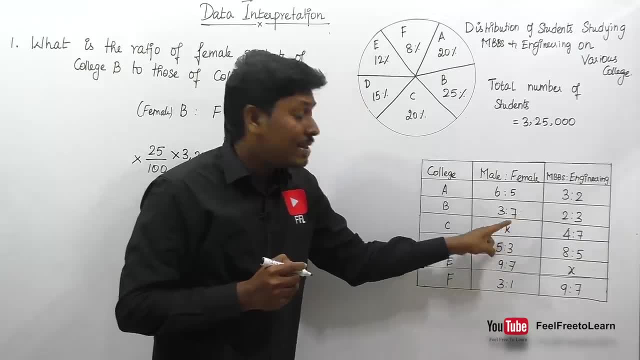 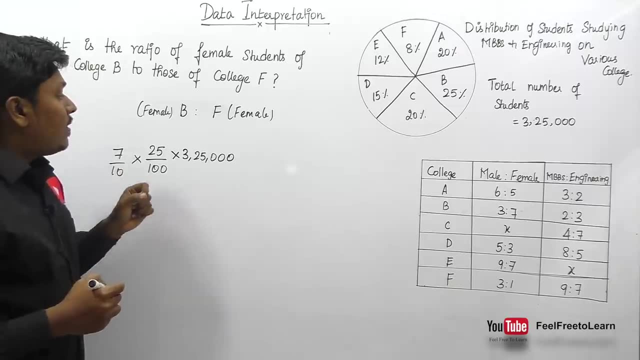 So, friends, college B, female are in a ratio 3 is to 7, that is 7 is the female ratio. So 7 divided by total ratio, that is 10.. So, friends, clear on the concept. Okay, Our next target to find the college F, female. Similarly, out of this, 2 lakh, that is 3 lakh, 25,000 students. 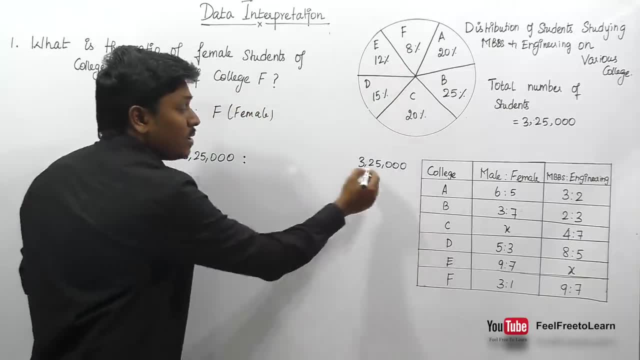 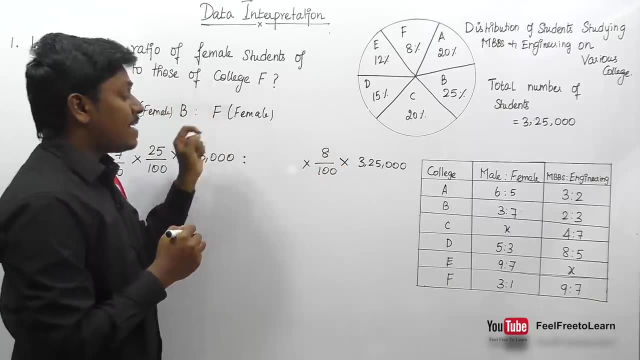 What about college F friends? College F is 8 percentage. So out of this 3 lakh 25,000 students, 8 percentage of students are in college F. So our target to find college F female. So college F female will be in the ratio male is to female, that is, 3 is to 1. Our target 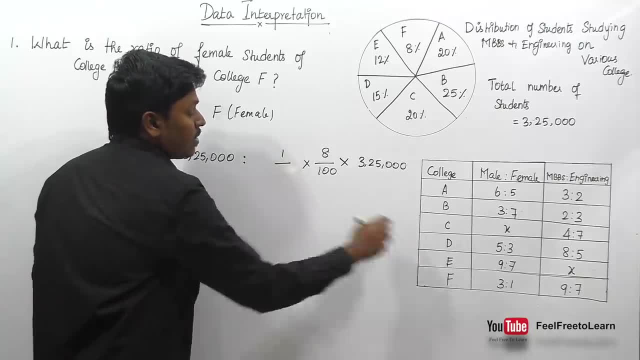 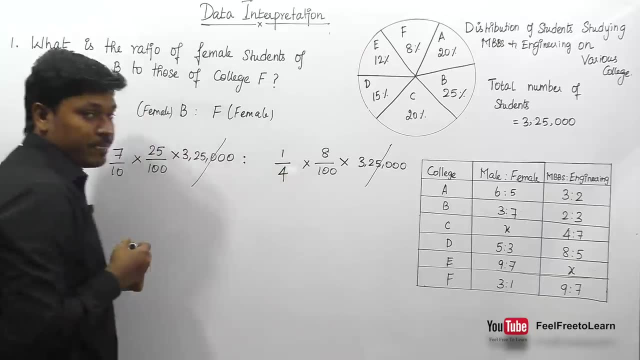 to find only female. So our target to find the college F, female is to female. that is 3 plus 1.. So we can cancel this 3 lakh 25,000 and 3 lakh 25,000. And similarly we can cancel this 100 and we can. 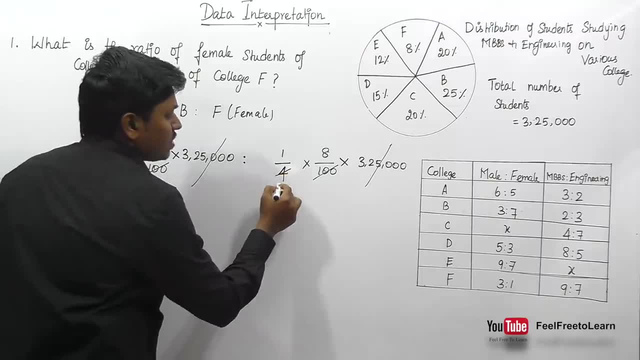 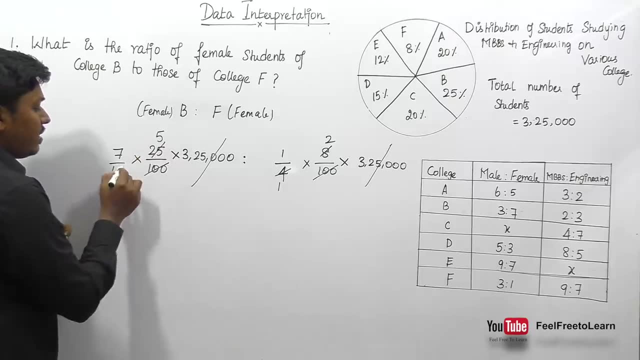 also cancel this 100.. So finally, we can cancel 1 4's are 4,, 2 4's are 8.. Okay, And I think we can cancel this 5 table. If I cancel this on 5 table, 5 5's are 25, 2 5's are 10.. I. 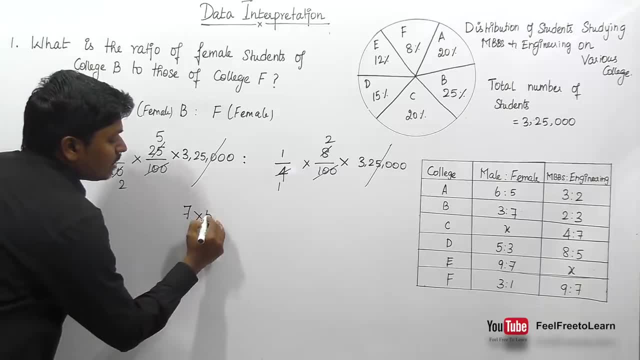 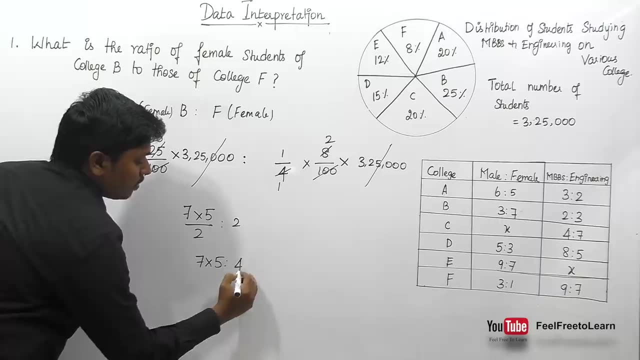 think we can't able to cancel any value. So the remaining are 7 into 5, divided by 2 ratio, Here it is 2.. So we can say that 7 into 5 is 2 into 2 will be 4.. So finally, 7: 5's are 35. So the ratio, 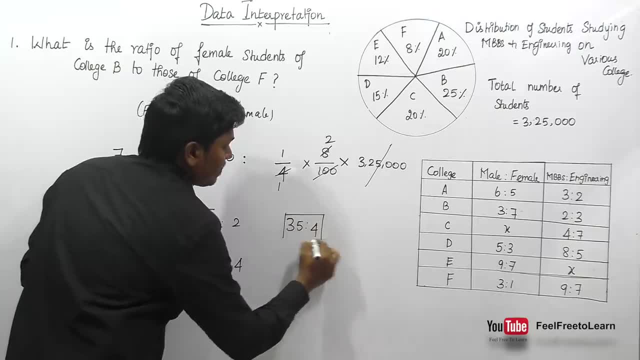 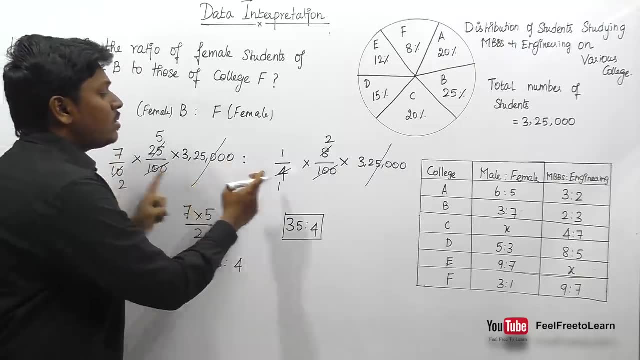 will be 35 is to 4.. So, friends, finally we got the ratio, that is, 35 is to 4 for question number 1.. So, friends, remember that don't calculate the value separately and don't calculate this value separately, And then some students will use to find the ratio. So don't do that in. 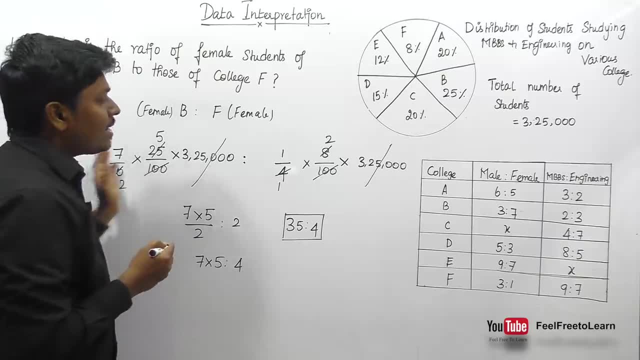 your exams. Always you should be faster. So the better thing, right in a single step, so that we can cancel all the values easily. Question number 1.. So we can cancel all the values easily. Question number 2.. So we can cancel all the values easily. Question number 1. So we can. 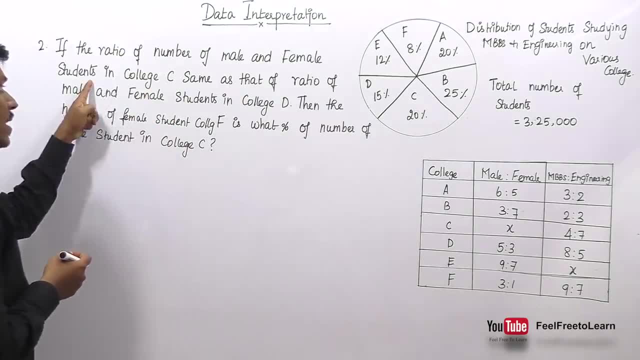 cancel all the values easily. Question number 1.. So we can cancel all the values easily. If the ratio of number of male and female students in college C is same as yet the ratio of male and female students in college D, Then the number of female student in college. 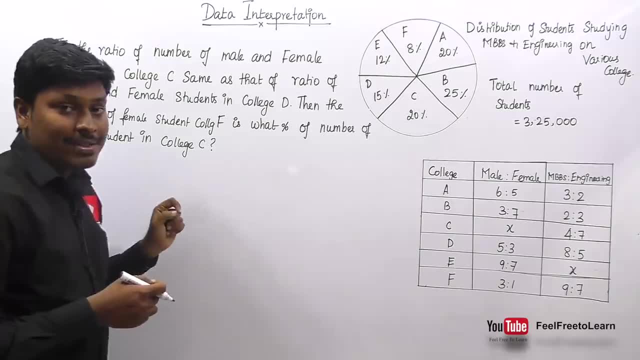 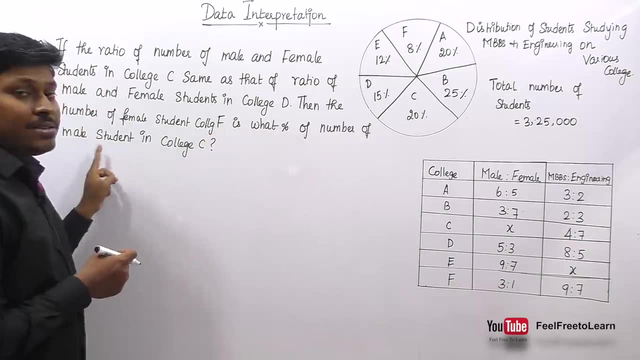 F is what percentage of number of male student in college C. So, friends, our target to find the female student in college here is what percentage of male student in college C. So, friends, always remember this. If in any where else in the data interpretation topic, if, 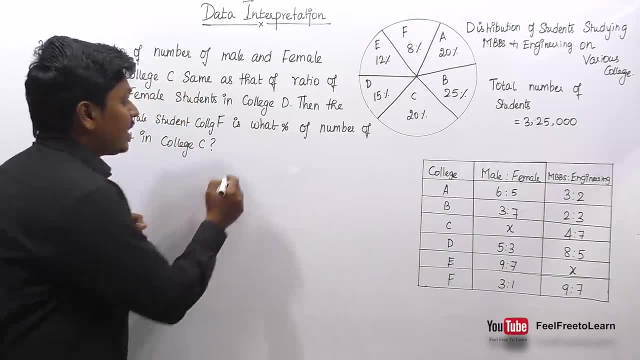 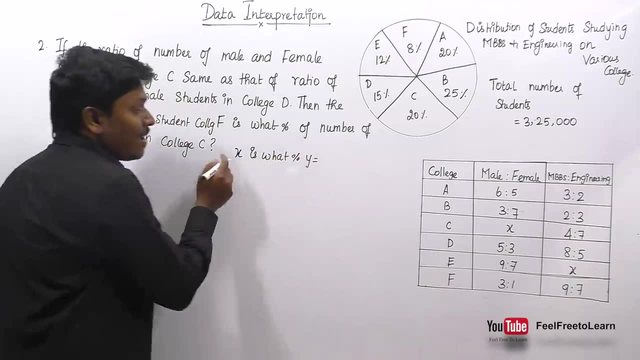 you find is what percentage, then definitely. we can say that the question in the format called x is: what percentage of y? in many of my videos i have told you that x is what percentage of y. that is x divided by y into 100. so, friends, here is what percentage of. if you find this word, then definitely. 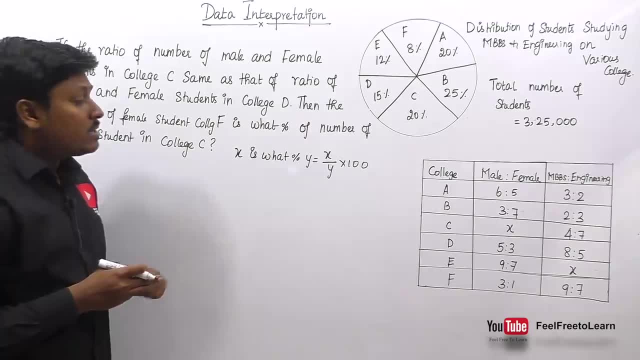 it will be in the format called x is what percentage of y. so, friends, the numerator x is the female student in college f and the denominator y that is male student in college c. but before that they have given a three points: the ratio of number of male and female student. 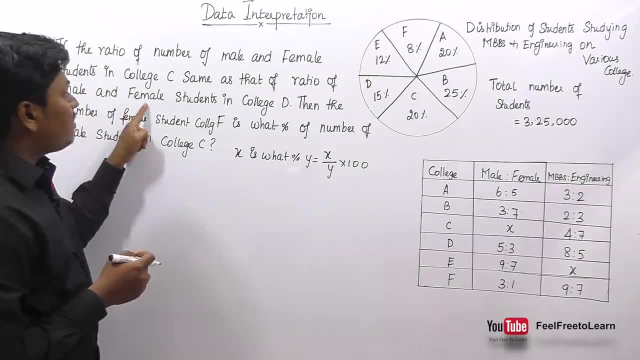 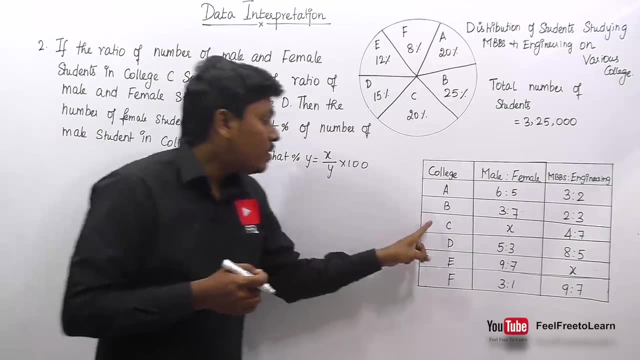 in college c is same as that of ratio and female, that is, male and female. students in college d. friends, listen carefully. here they have given a table chart. in the table chart we don't know the college c male and female ratio, but in the question they have given a clue that both c and d 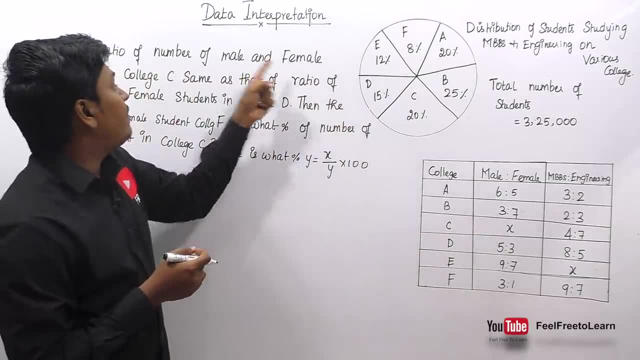 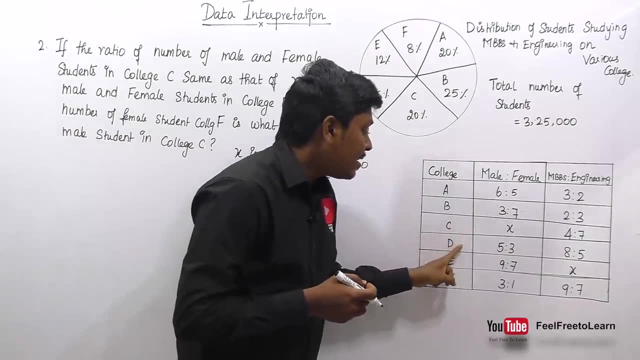 male is to female ratio will be same. see, friends, male and female ratio. college c is same as that of the college d male and female ratio. so So we can surely say that this college C and college D, both the male and female ratio, are same. 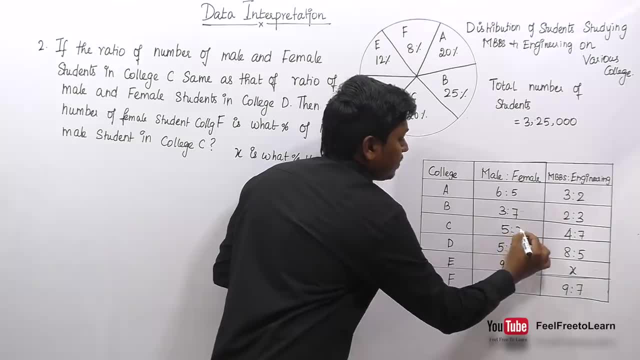 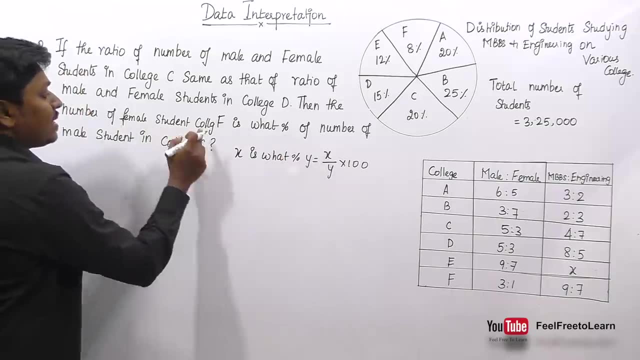 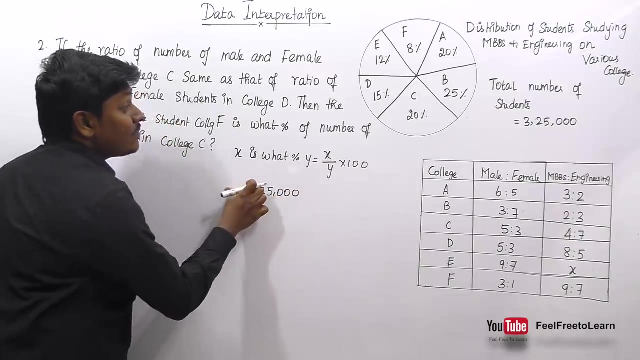 So we can surely say that this X will be 5 is to 3.. Okay, So, friends, let me find this X is what percentage of Y? Okay, The numerator X, that is, female students in college? F. So, friends, out of this 3,25,000 students, how many students are there in college F, friends? 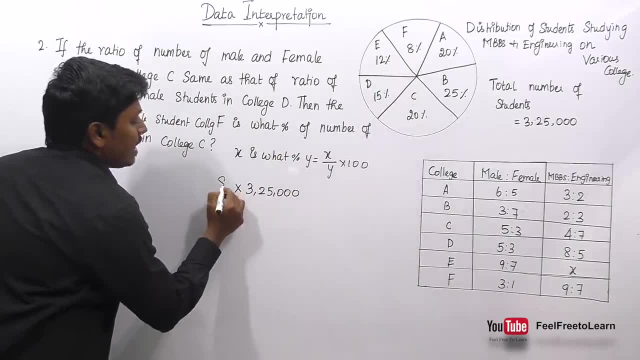 So the college F, which has 8 percentage. So we can write this as 8 divide by 100.. So out of this, 3,25,000 students, college F. that is 8 by 100, that is 8 percentage. 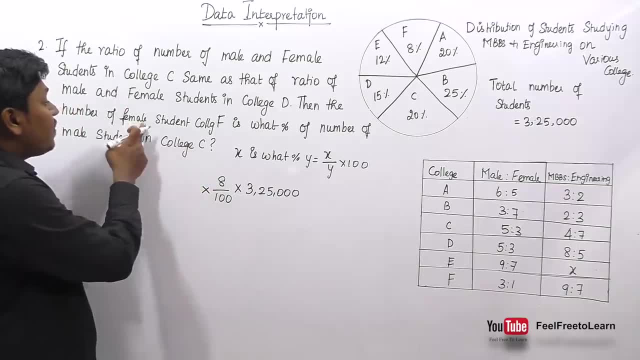 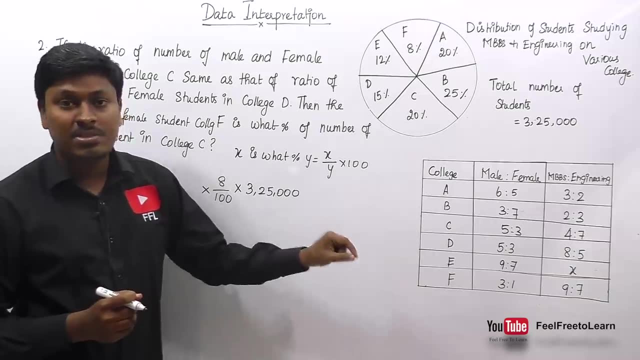 So out of this 8 percentage we have a target to find only female in college F. So the college F female are in a ratio 3 is to 1, that is male and female ratio 3 is to 1. Our target to find only female. 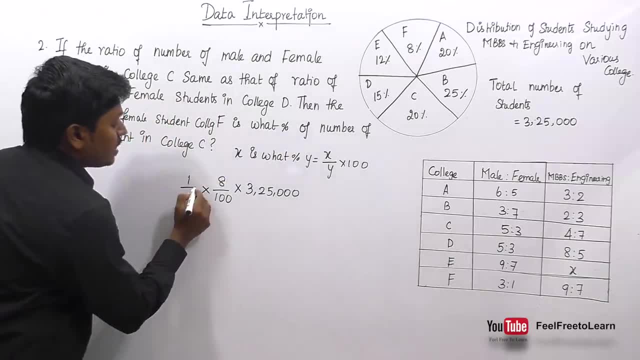 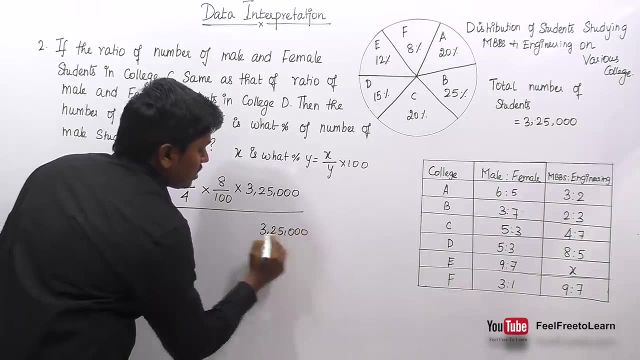 So females are in a ratio 1.. So 1 divided by the total ratio, that is 4.. Okay, Divided by next step. So out of this, 3,25,000 students. So out of this, 3,25,000 students. 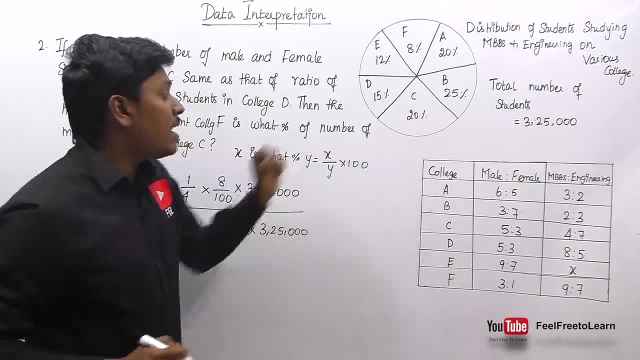 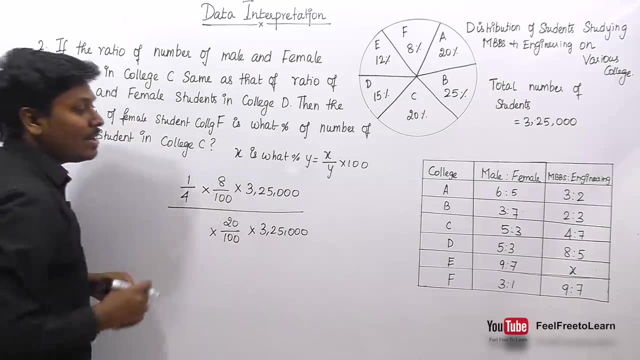 So how many students are studying in college C? So, friends, the college C are in a ratio, 20 percentage, that is 20 divided by 100.. So into our target to find the male students in college C. So the college C male and female ratio 5 is to 3.. 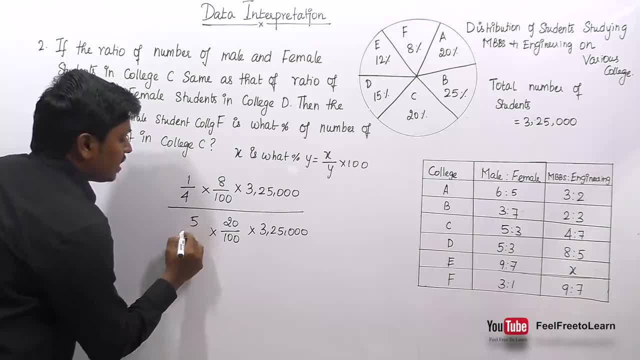 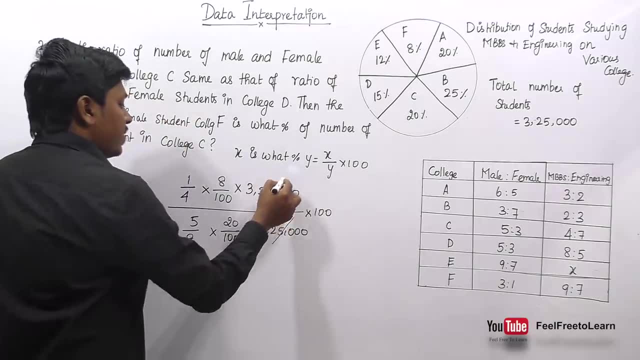 The male ratio are 5.. So 5 divided by the total ratio, that is 8 into 100.. So this looks like a format called X divided by Y into 100. So we can cancel this: 3,25,000, 3,25,000.. 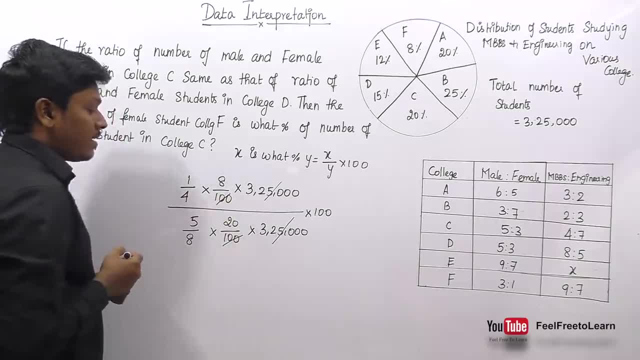 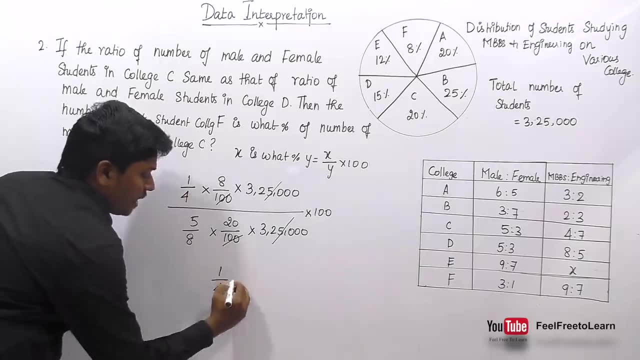 And similarly we can cancel this 100 and we can also cancel this 100.. Okay, I think we can cancel this or write the next step, friends. So the remaining values are 1 by 4 into 8.. Right, So divided by here, the remaining values are 5. divided by 8 into here, it is 20.. 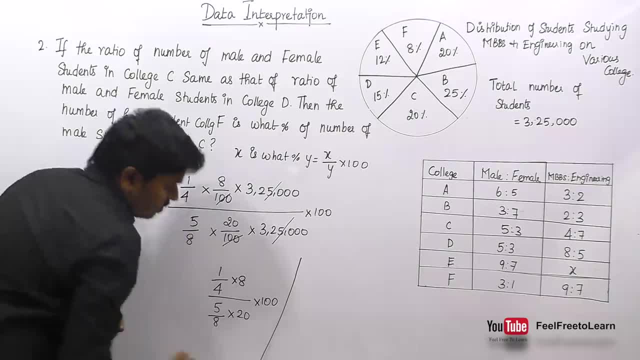 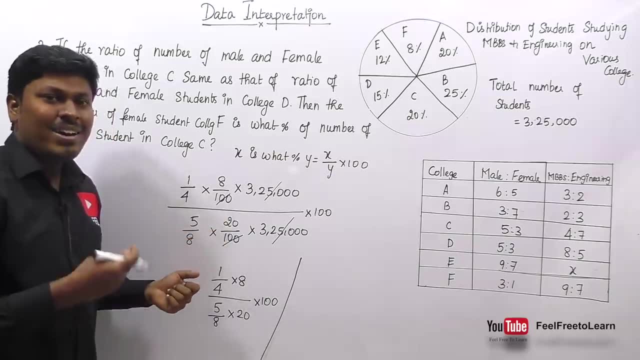 So into 100.. So, friends, if you are a brilliant, you can directly cancel 4 into 2, will be 8. And we can cancel this on 2 table. Right, If you are a beginner. So write this step, but don't write this in your exam. 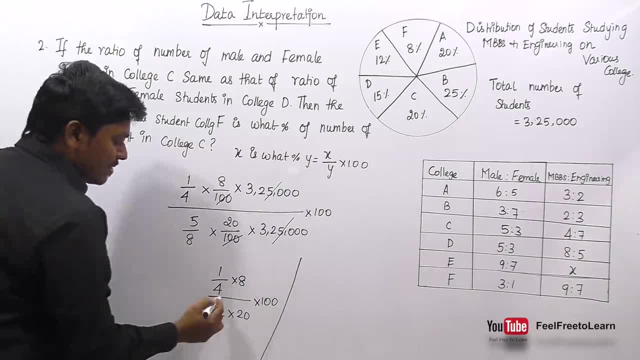 Right For a practicing. you can write these Now: when we cancel this, 1: 4's are 4, then 2: 4's are 8. And I think we can cancel this on 4 table 2 times. If I cancel this on 4 table, that is 5 times. 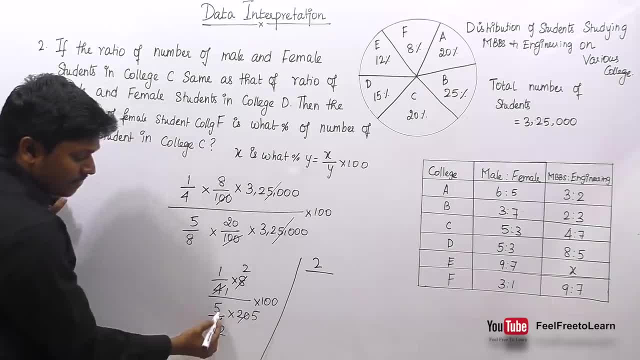 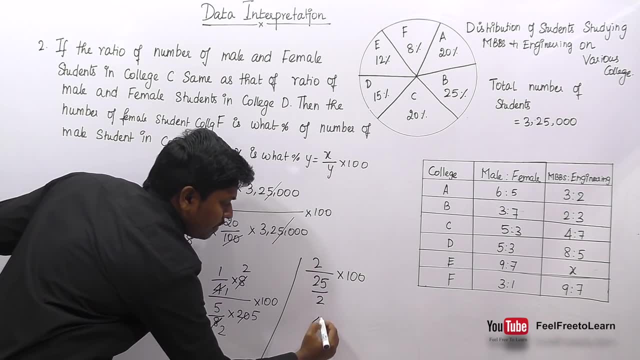 So finally, the numerator we have 2. And the denominator we have 5.. 5 into 5 will be 25, friends, And the denominator we have 25.. So we can write this as: 2 into 2 will be 4 divided by 25 into 100.. 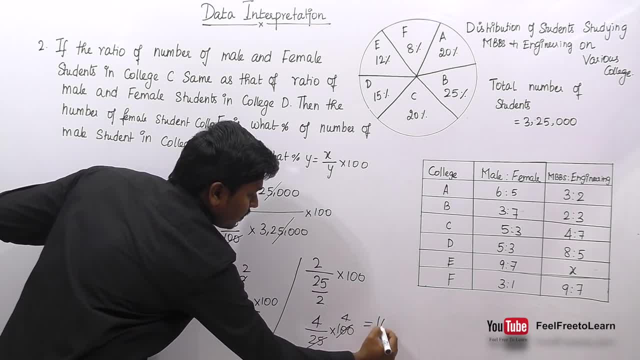 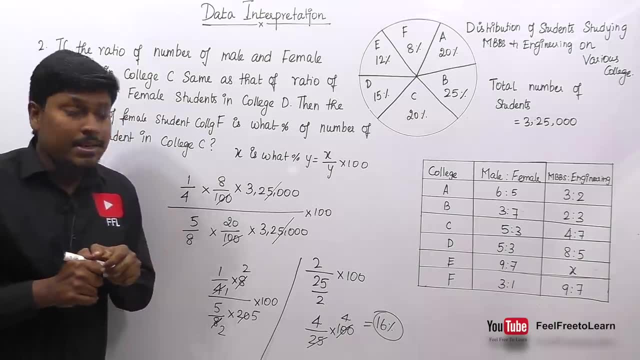 So when we cancel 25 4 times, So 4 into 4 will be 16.. So finally we got the answer: 16 percentage for question number 2.. So friends always remember that if it is in the format anywhere else in the D equation. 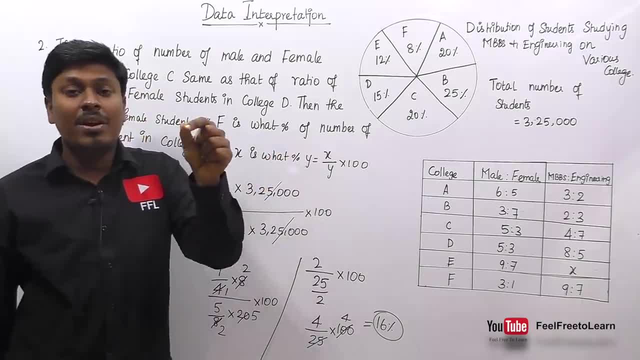 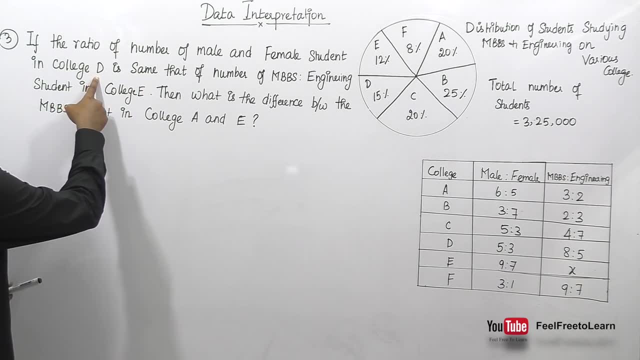 If you find x is what percentage of y, Then it will be the formula called x divided by y into 100.. Question number 3.. If the ratio of number of male and female students in college D is same that of number of MBBS and engineering students in college E, 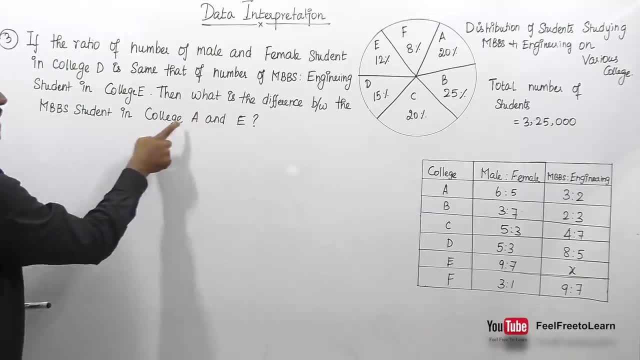 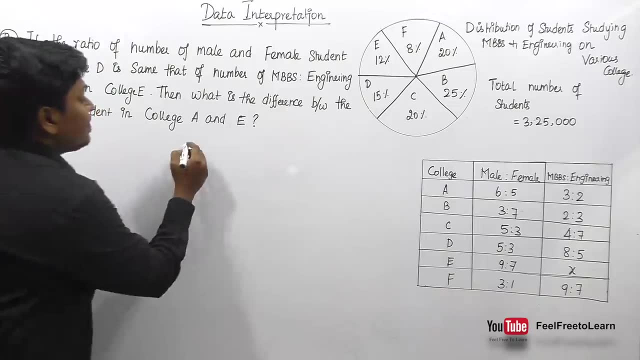 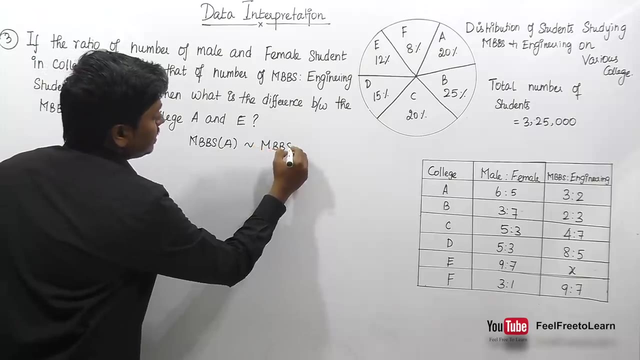 Then, what is the difference between the MBBS students in college A and E? So, friends, our target: to find The difference right. that is difference for the MBBS students. So, friends, we need to find the difference for MBBS students in college A to the MBBS students in college E. 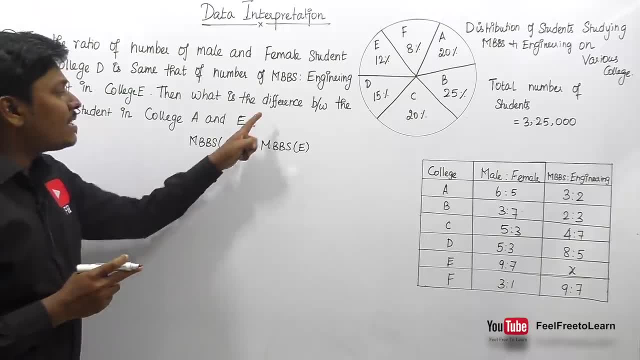 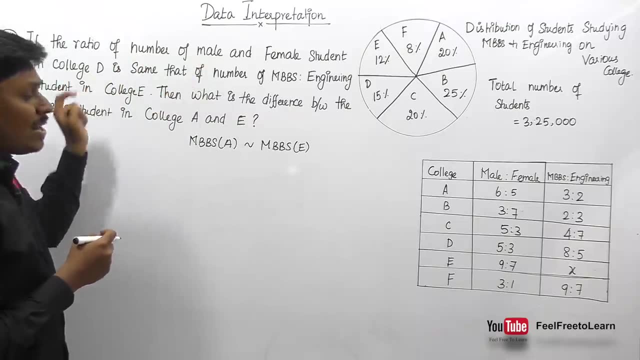 Okay. So this is our target, friends, We need to find the difference, Difference, that means subtraction, right, Okay, But they have given a clue: that ratio of number of male and female students in college D- Okay. So, friends, see here, friends, college D male and female ratio are 5- is to 3.. 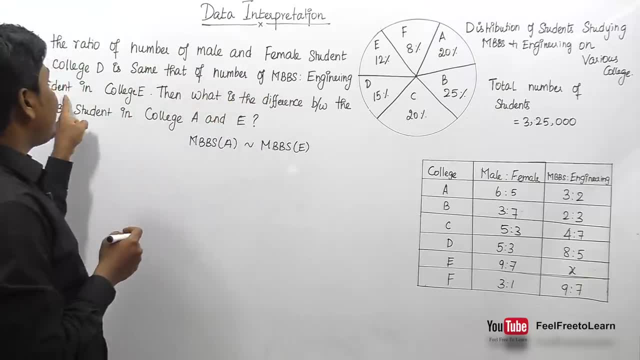 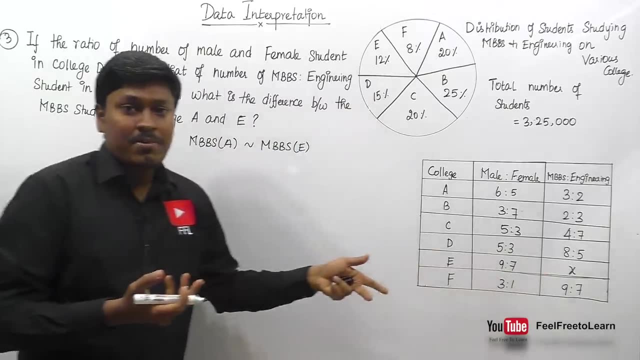 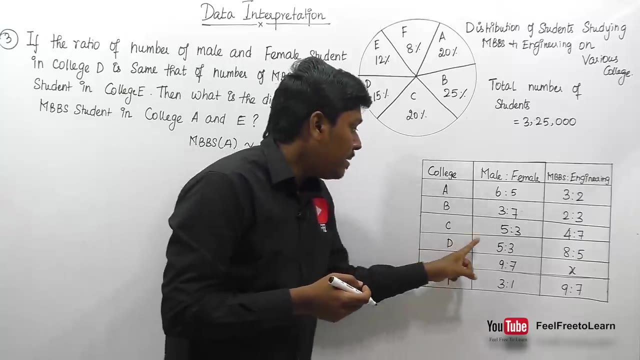 Okay, Is same as that of number of MBBS and engineering students in college E. Friends, listen carefully. in college E we don't know what is how. what is the students number of students who are there in MBBS and engineering? But here in the question they have given a clue. that is, the college D male and female ratio is same as that of MBBS and engineering in college E. 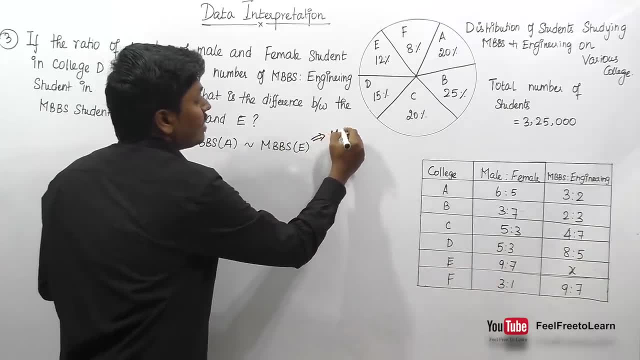 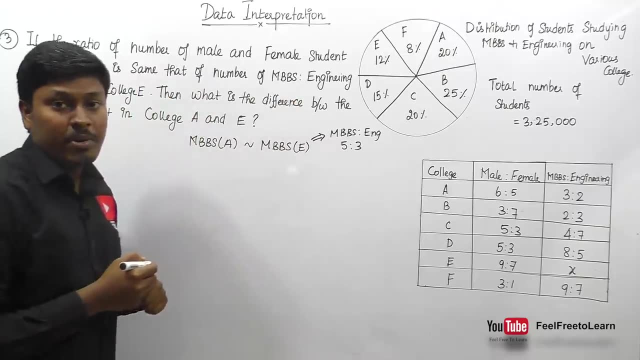 So we can say that the college E MBBS and engineering are in a ratio that is 5 is to 3.. So this is the clue they have given in the first three points. and the next point: we need to find what is the difference between MBBS in college A and MBBS in college E. 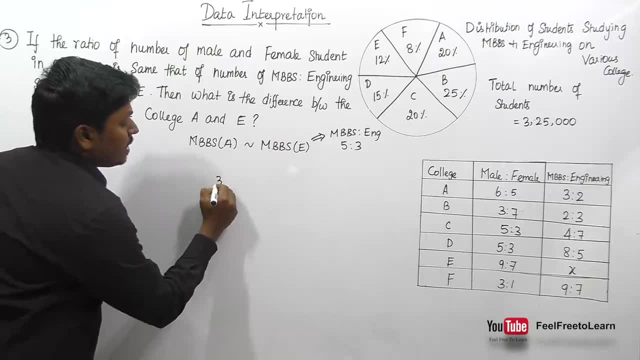 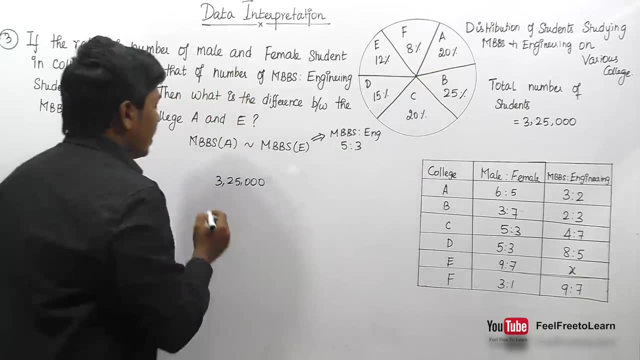 Okay, friends, we know that, first of all, total students are 3,25,000.. So, out of this 3,25,000, see how many students are studying in college A. So the college A, the number of students, will be 20, percentage, that is, 20 divided by 100. 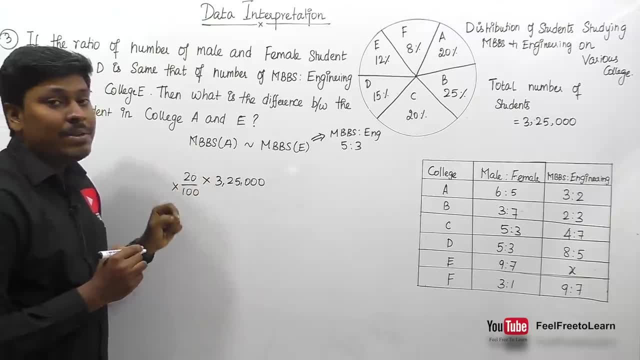 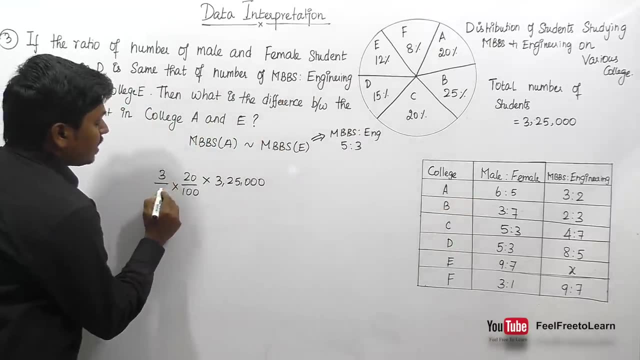 Okay, Out of this 20 percentage, our target to find only MBBS in college A, So the college A, So the college A MBBS students are in a ratio 3.. So 3 divided by the total ratio, that is 5.. 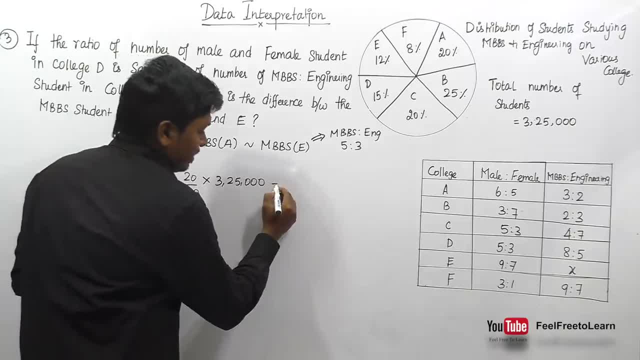 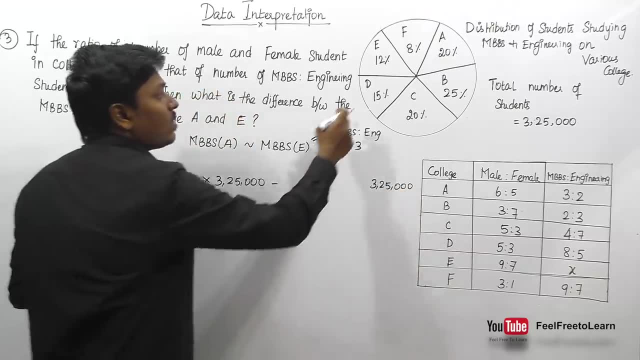 So 3 plus 2, the total ratio 5.. So difference, that means subtraction. Similarly, out of this 3,25,000 students. So how many students are there in college E? So college E is 12 percentage. 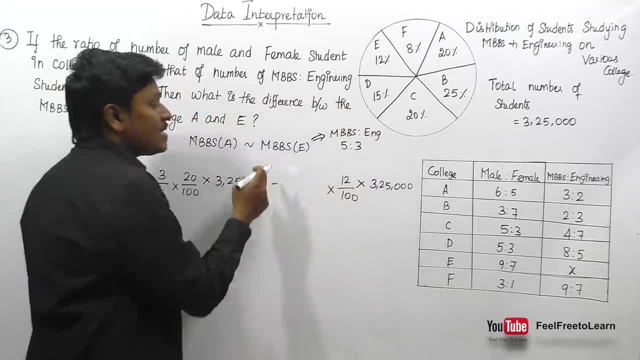 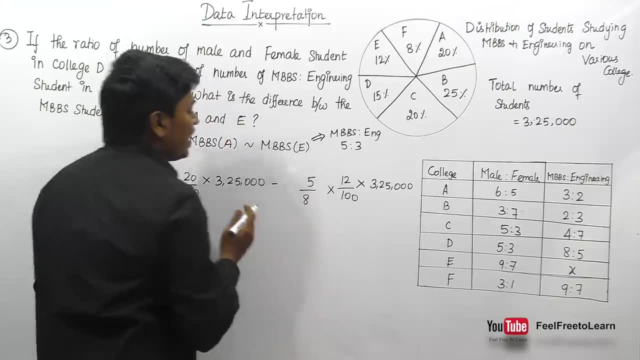 So 12 divided by 100. So out of this 12 percentage, our target to find that is MBBS. So, friends, MBBS are in a ratio that is 5 and the total ratio that is 8.. So we need to calculate this. 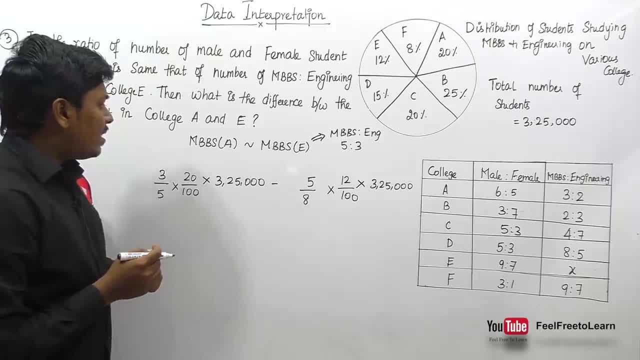 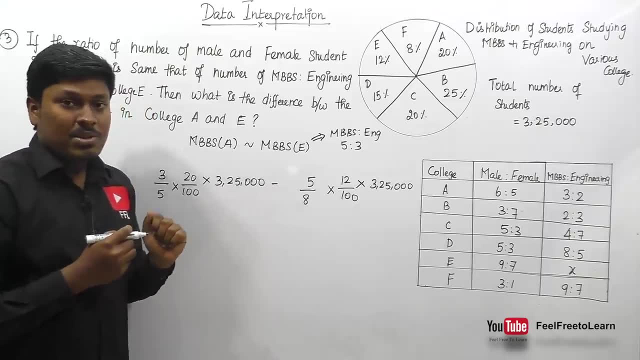 And we need to find that difference. Friends, always remember that if it is a ratio, we can cancel this 23,25,000 and 3,25,000. But here we need to subtract this. So, friends, do one thing: Don't separately calculate left hand side part and right hand side part. 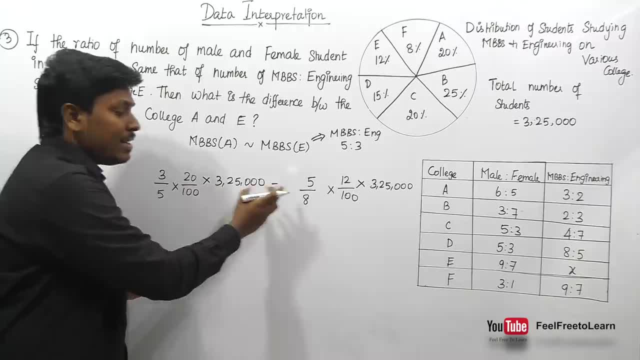 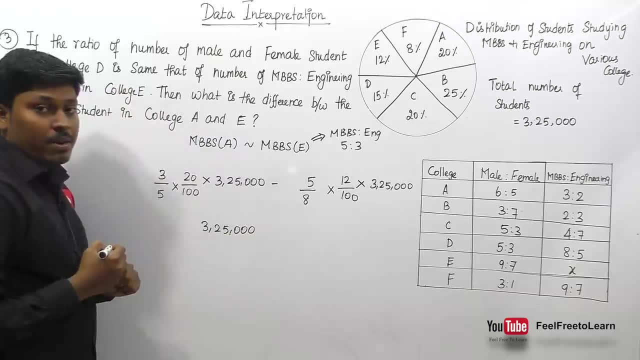 Then don't go for the difference. Here 3,25,000 and here 3,25,000 is common, So let me take 3,25,000 from both these values common. Okay, Next step. here we can find 100 and here we can find 100.. 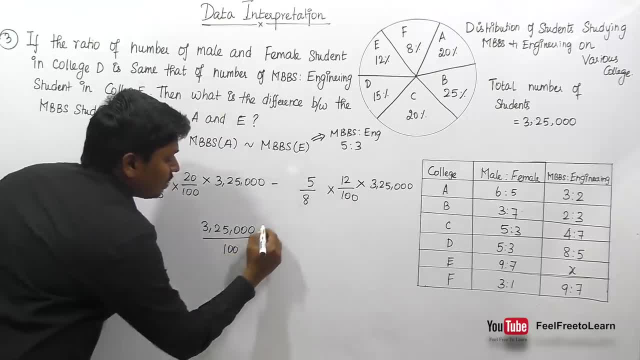 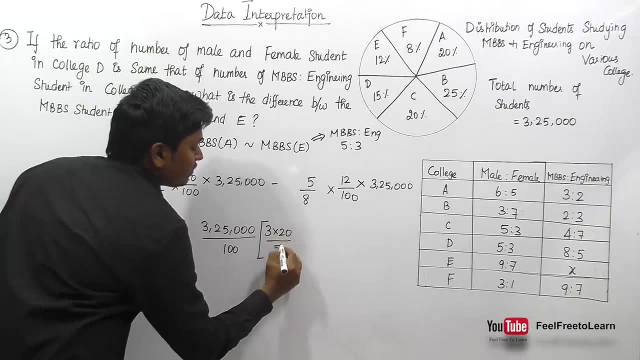 So similarly, from both the numbers we can take 100 as common. So the remaining numbers are 3 into 20 by 5.. So 3 into 20 divided by 5. And here 5 into 12.. So 5 into 12 divided by 8.. 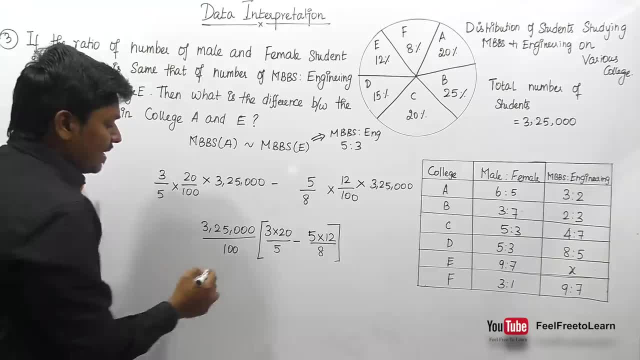 So these are the numbers are remaining. So, friends, now I think we can cancel this 0,0 and we can cancel this 0,0.. So here we have 3,000, that is sorry. Here we have 3,250.. 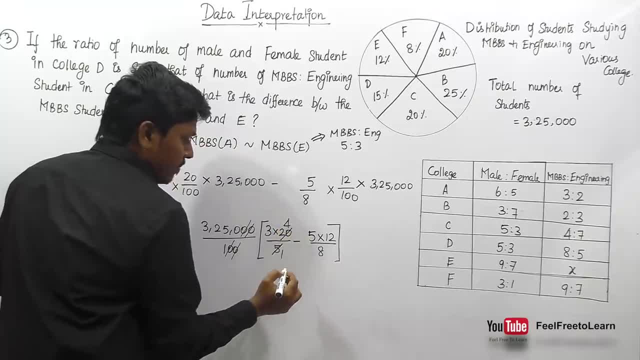 So try to cancel this 1,5,5.. 5,4 are 20.. So similarly, we can cancel this on 4 table. If I cancel this on 4 table, 4,2 are 8.. 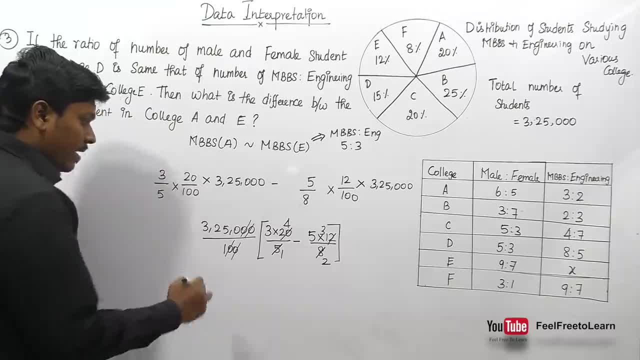 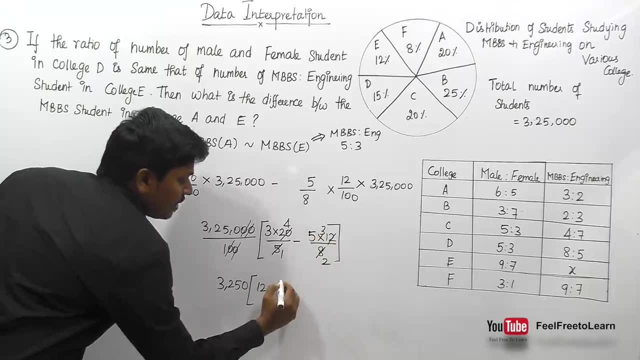 4,3 are 12.. I think we can't able to cancel anything. Okay, Finally, we got 3,250.. That is, 4 into 3 will be 12.. So here, 5 into 3 will be 15.. 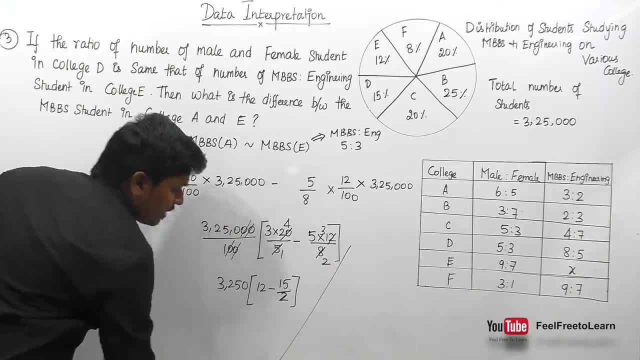 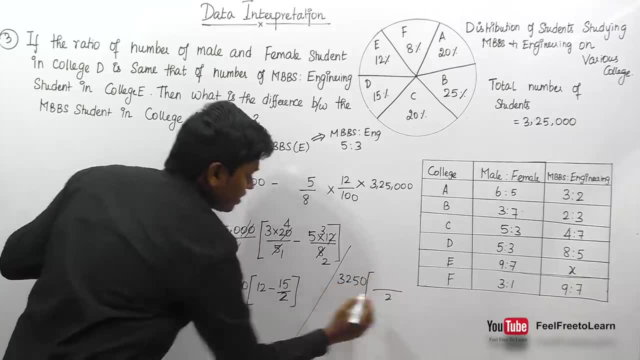 15 divided by 2 friends, So this can be written as 3,250.. So 3,250.. So let me take LCM as 2.. So if I take LCM as 2.. 12 into 2 will be 24.. 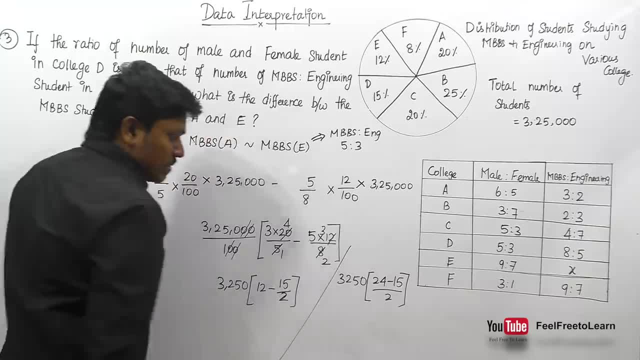 So 24 minus 15 divided by 2.. So I think we can cancel this on 2 table. friends, If I cancel this on 2 table, 1,2's are 2.. Remaining will be 1,, 6,2's are 12.. 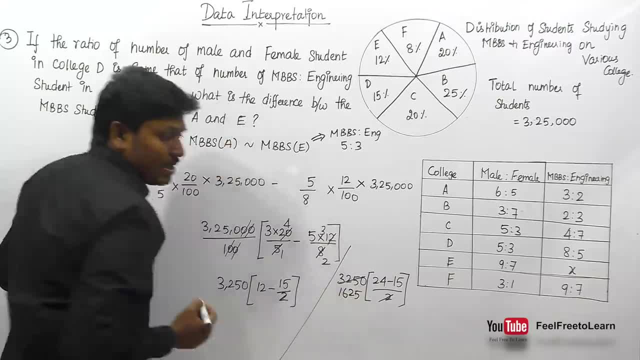 Remaining will be, that is, 2,2's are 4.. Remaining will be 1,, that is 4.. So finally we can say that 1,6,2,5.. So 24 minus 15 will be 9.. 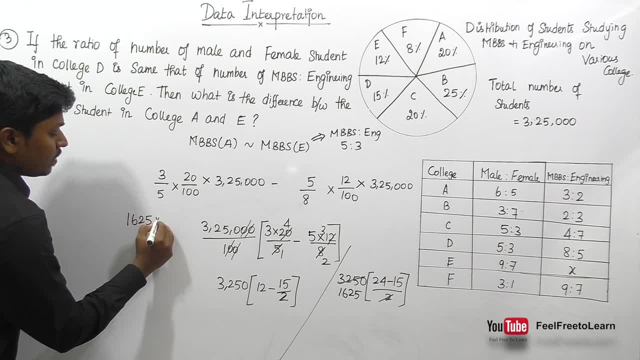 So, finally, we need to multiply, that is, 1,6,2,5 into 9.. So, friends, 9,5's are 45. The remaining will be 4.. So 9,2's are 18 plus 4 will be 22.. 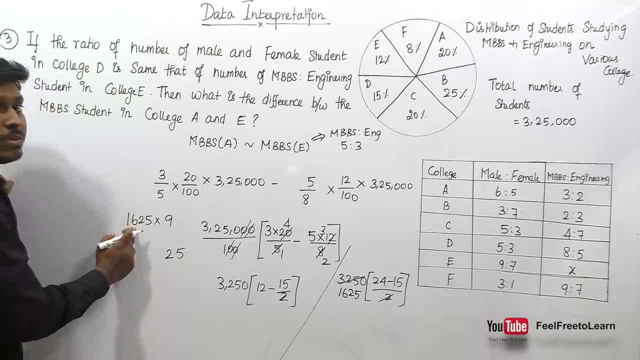 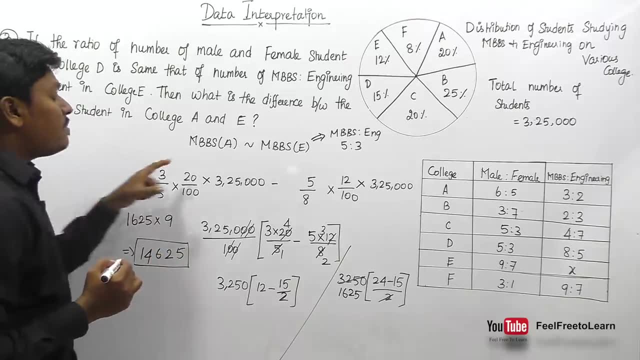 The remaining will be 2.. So 9,6's are 54.. 54 plus 2 will be 56.. The remaining will be 5.. So 9,5, that is 14.. So finally we can say that the difference for MBBS in college A and difference in MBBS for college E, that is 14,625.. 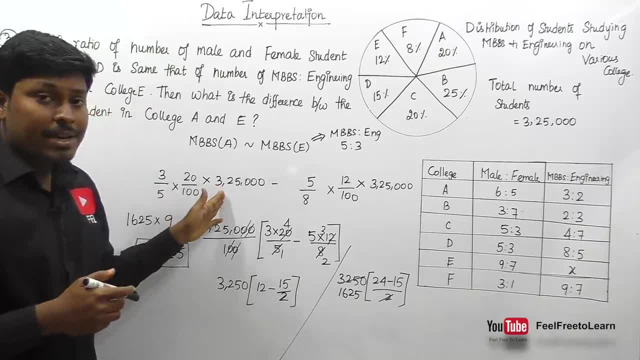 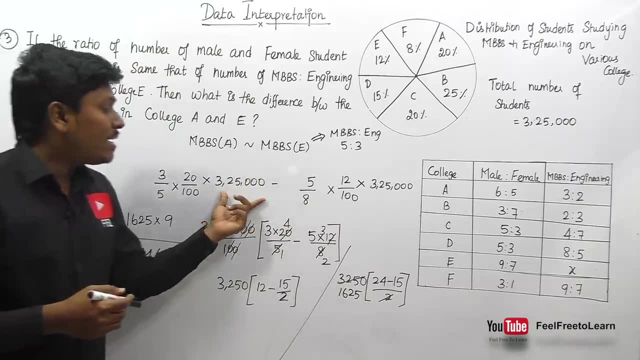 So friends always remember that don't find the left hand side parts separately and right hand side parts separately. That will make you more than 1 or 1 and half minute. So if you need to solve the question faster, In both the cases where we can find 3,25,000 common 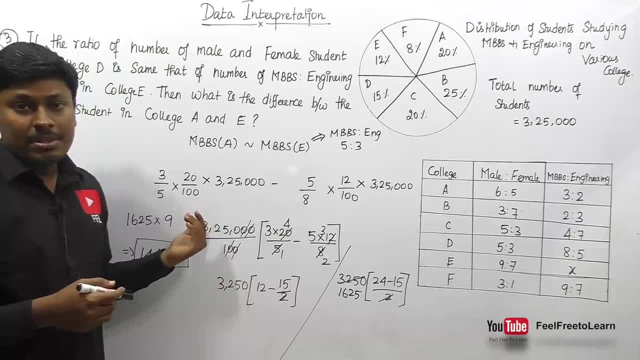 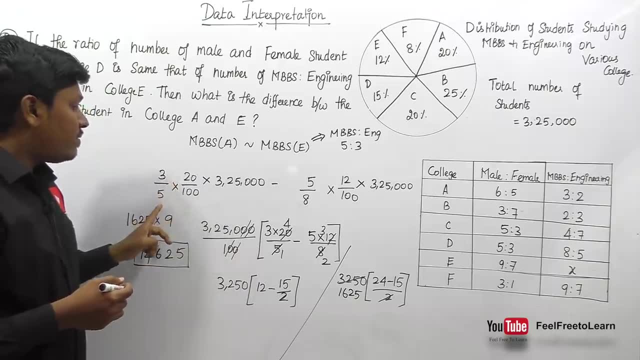 So just stay focused. Take 3,25,000 common from both these numbers. Similarly we can see here also 100 and here also 100. So I have took 100 as common. So the remaining numbers 3 into 20 divided by 5.. 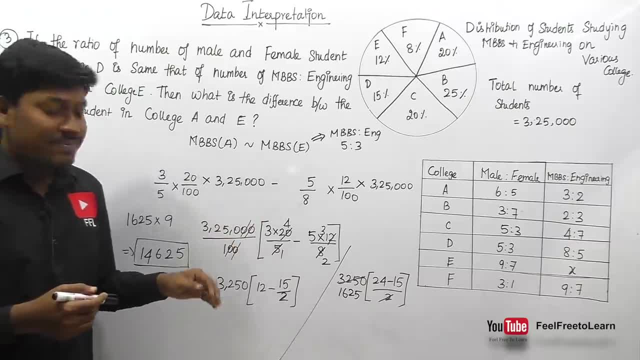 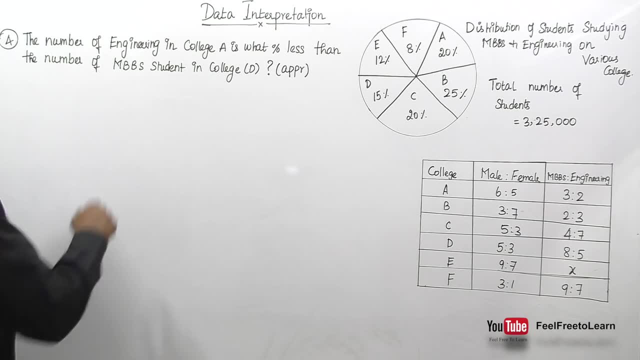 So 5 into 12 divided by 8.. So after simplifying this, finally we got the answer, that is 14,625 for question number 3.. Let me move on to the last fourth question. The number of engineering students in college A is what percentage less than the number of MBBS students in college D? 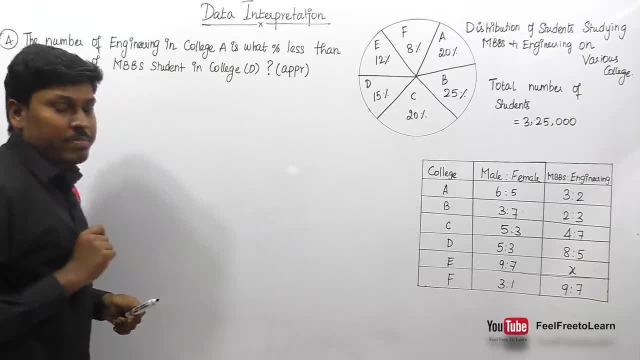 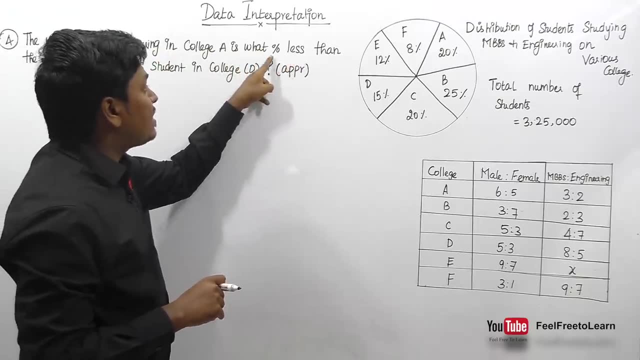 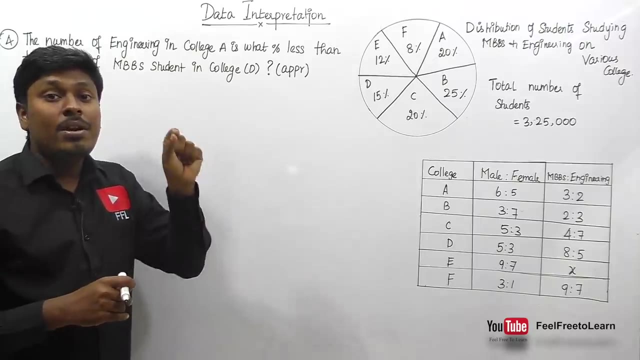 That means we need to find an approximate value. Friends, listen carefully. Our target to find the total number of engineering students in college A is what percentage less, Friends listen carefully, Is what percentage less According to question number 1.. If the question is in the format called, x, is what percentage of y? 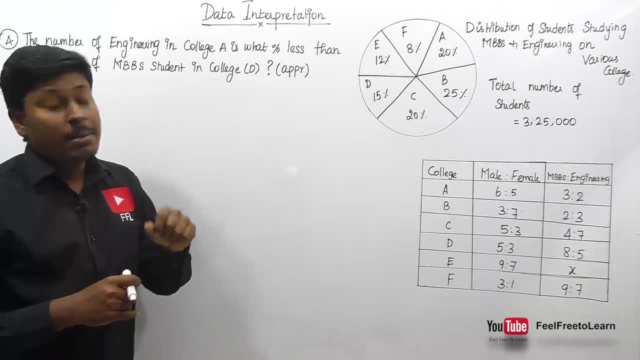 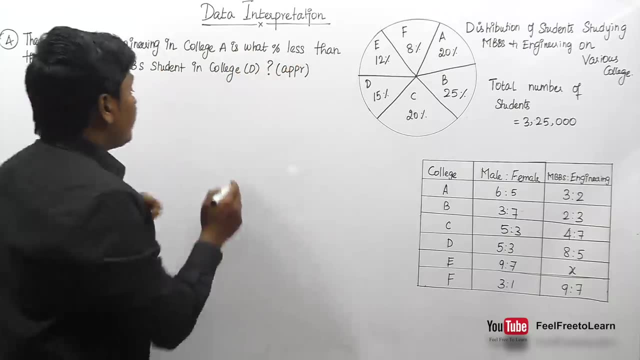 Then we use a formula called x divided by y into 100.. But here it is similar, But here they have given an extra word, that is: x is what percentage less. So we should use a formula that is: x is what percentage less. 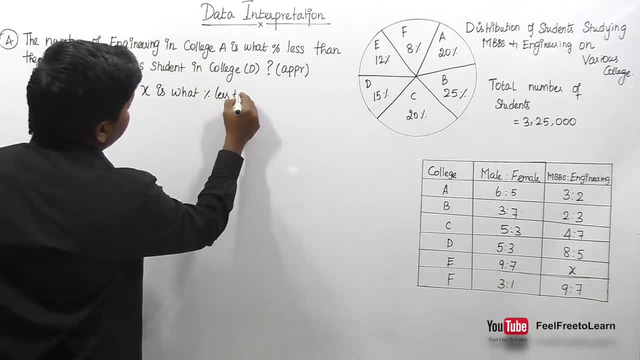 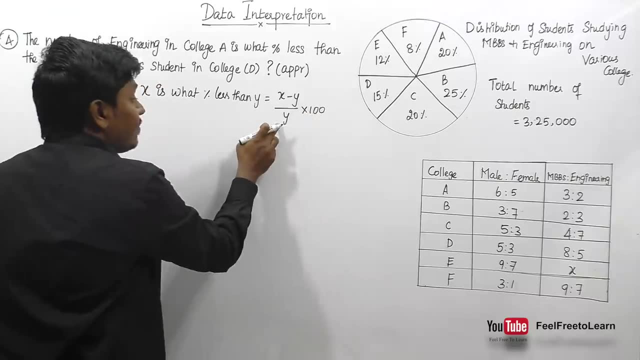 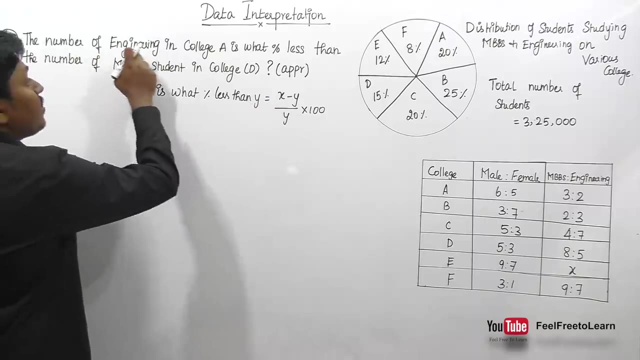 What percentage? less than y. So then the formula is x minus y, divided by y into 100.. So, friends, listen carefully, The denominator y will be MBBS students in college D And the value of x, that is numerator, the total number of engineering students in college A. 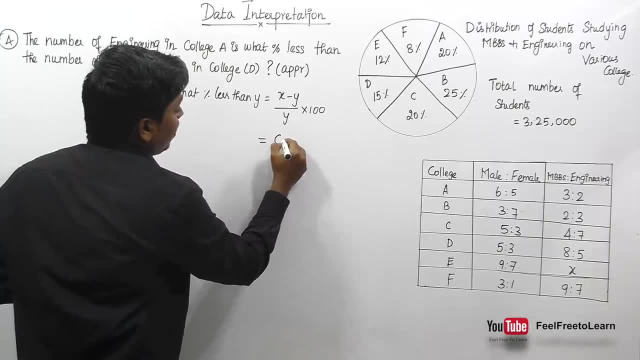 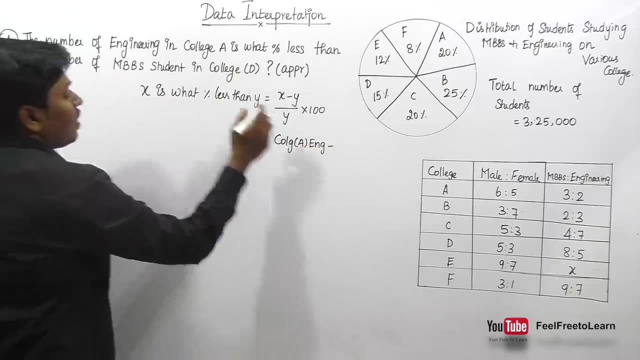 That is most important, friends. So we can write this. So college A engineering. So minus the y determines MBBS: students in college D, So college D MBBS, So divided by. don't write this in your exams. 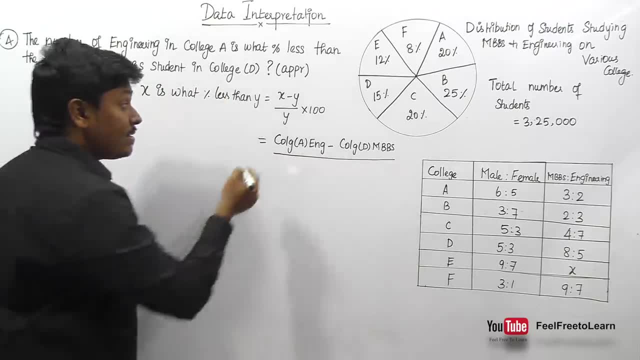 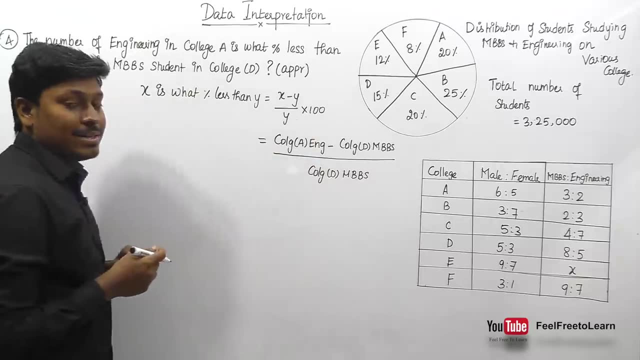 In order to understand you clearly, I am just writing these steps. So college D- MBBS. So we need to substitute all the values And we need to find how much percentage it is less. So, friends, our target to find engineering in college A: 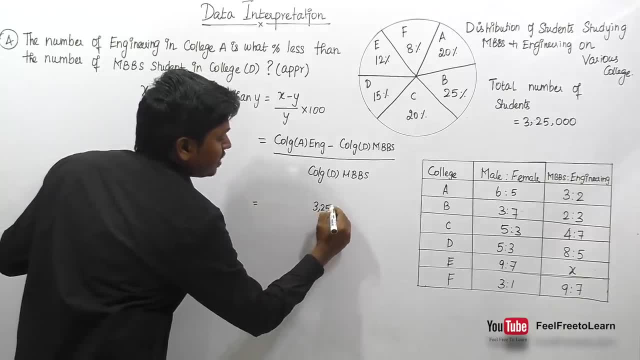 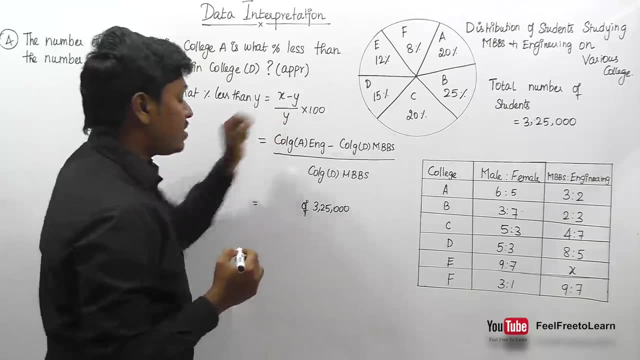 We know the total: there are 3,25,000.. So we can write this at 3,25,000.. So out of this 3,25,000 the college A is 20% friends. So 20 divided by 100 of that means multiplication. 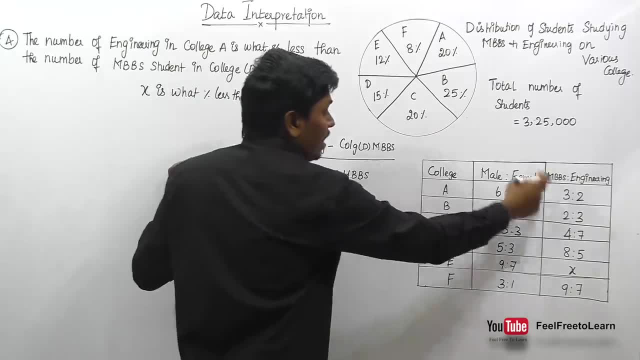 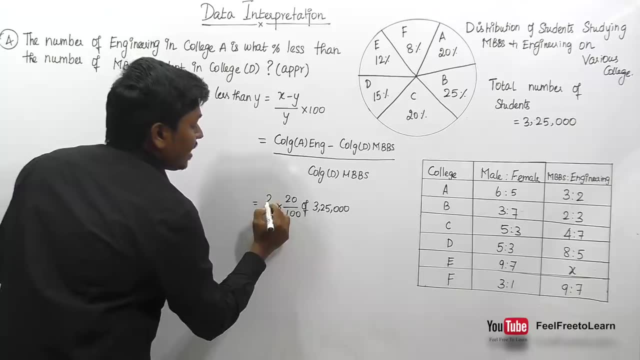 So, friends, our target to find engineering, So engineering in college A, The engineering in college A, that is 3- is to 2 ratio. So the engineering or 2 ratio, the total that is 5.. So we can write this as 2 divided by 5.. 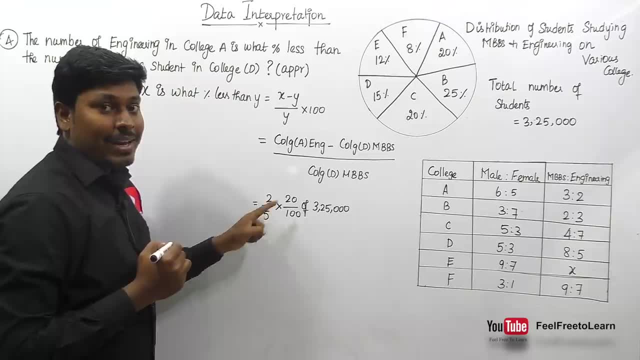 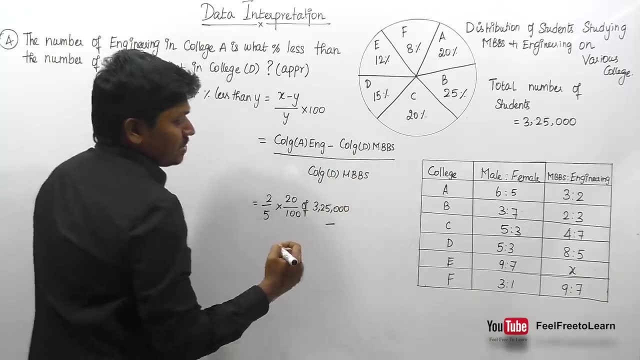 So, friends, college A engineering, that is 2 by 5 into 20, divided by 100 into 3,25,000.. So next is college A engineering. So next is college D, MBBS. So similarly, we have 3,25,000.. 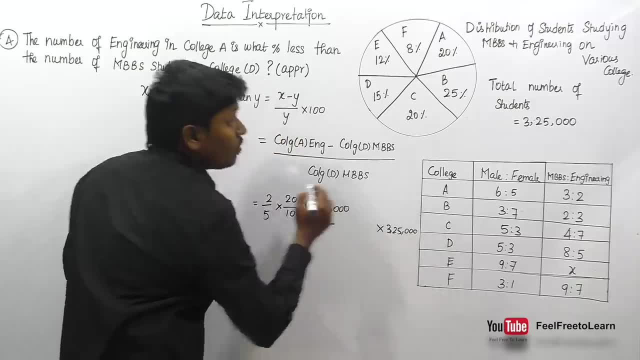 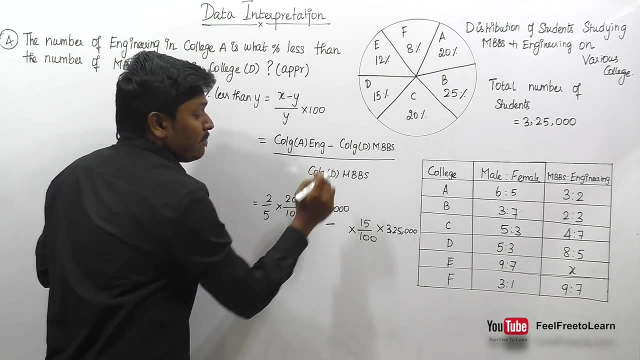 So out of this 3,25,000, we need to find how much students are studying in college D. So the college D is 15%. that is 15 divided by 100.. So we need to find the MBBS. 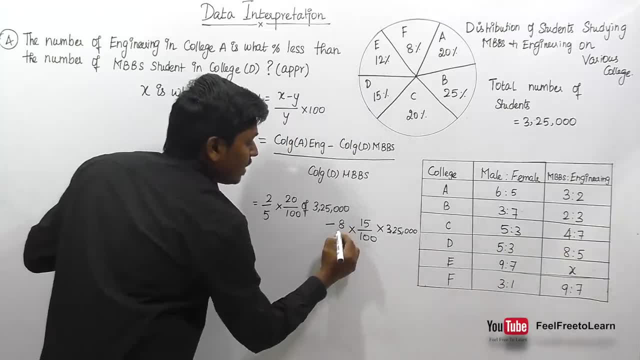 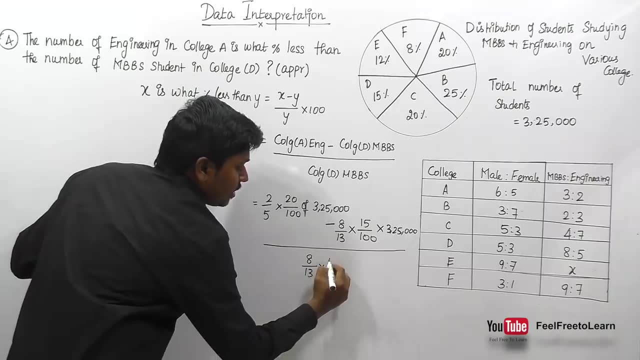 So college D MBBS are 8.. So 8 divided by total ratio, that is 13.. So divided by, So college D MBBS, that is 8 divided by 13 into 15, divided by 100 into 3,25,000.. 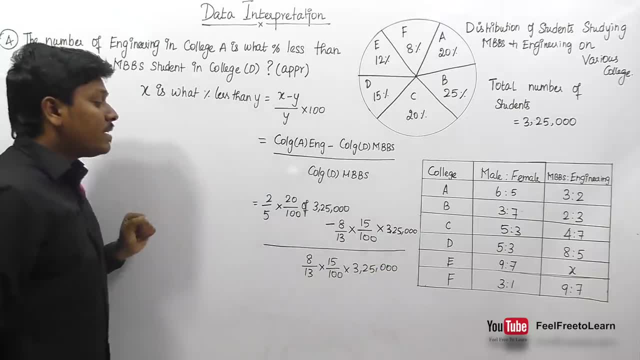 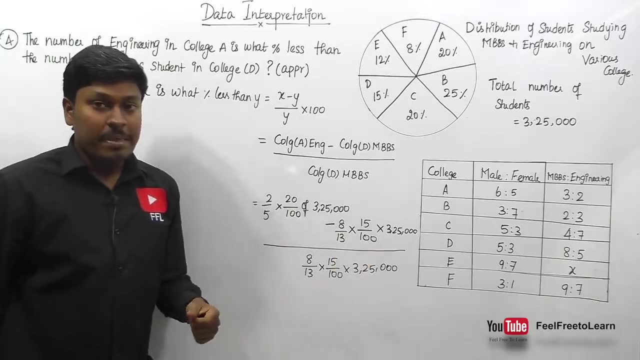 So, friends, remember that after writing this step, there is a huge calculation right. We need to find this value, then we need to subtract with this value, then we need to divide this value. Friends, my advice: in all the four terms, we can find 3,25,000 in common. 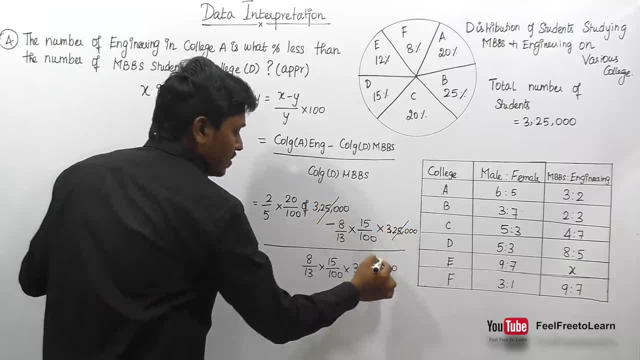 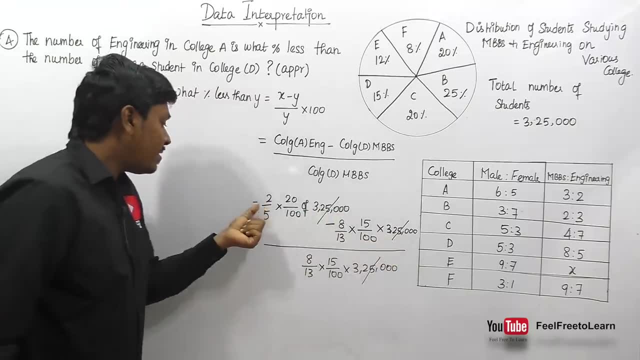 So we can directly say that we can cancel all the 3,25,000.. Friends got the logic in the numerator: here 3,25,000, here 3,25,000. from both the term we should take 3,25,000 as a common. 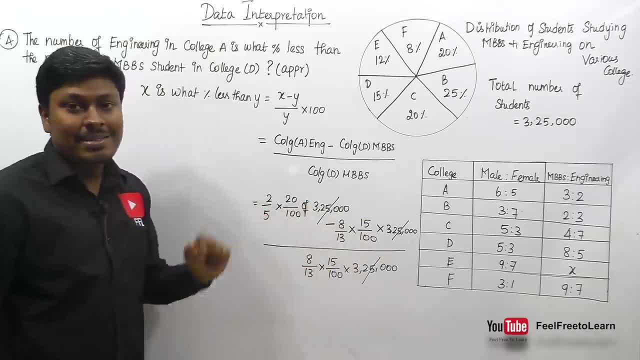 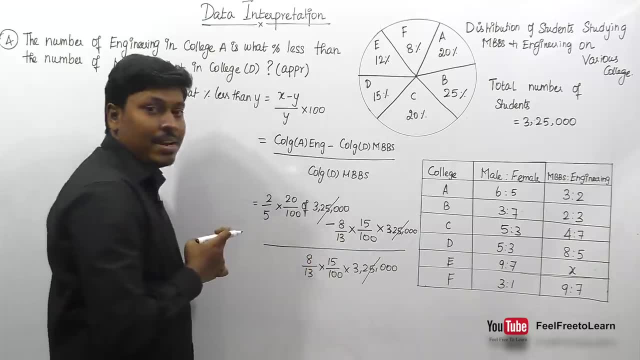 We can say that If all the term has 3,25,000, we can easily cancel it, right. Okay, Next step. See here, friends, in this term, where we can find 100.. Similarly, in this term, I can find 100, and in this term I can find 100.. 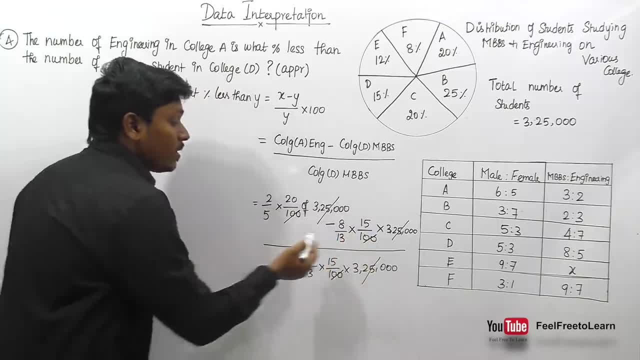 So I can say we can cancel all the 100 terms. right, Don't cancel 8 by 13,, 8 by 13.. Why? because in all the term the value should be 8 by 13. Here it is 8 by 13.. 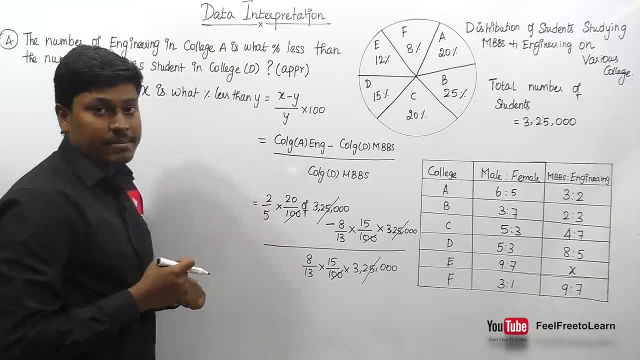 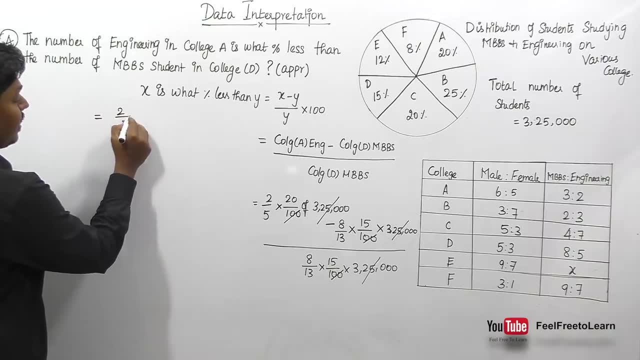 Here it is 8 by 13. But here we can't able to find 8 by 13.. So, friends, the remaining numbers are: that is 2.. Okay, I can write here. The remaining numbers are 2 divided by 5 into 20, minus of 8 divided by 13.. 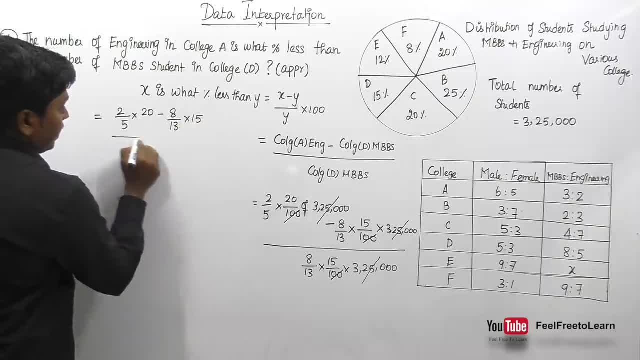 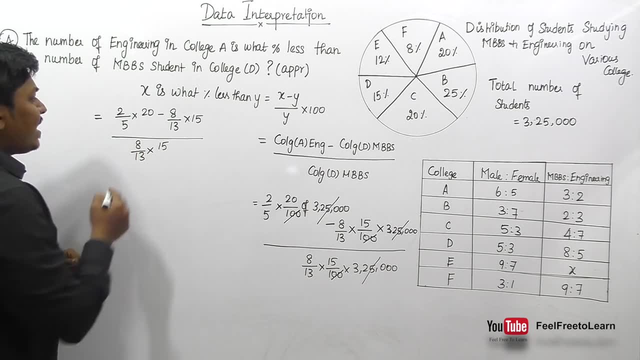 So 8 divided by 13 into 15.. So, divided by the remaining here, it is 8 divided by 13 into 15.. Okay, So, friends, I think we can cancel this on. Okay, Let me cancel this on 5 tables of 4 times. 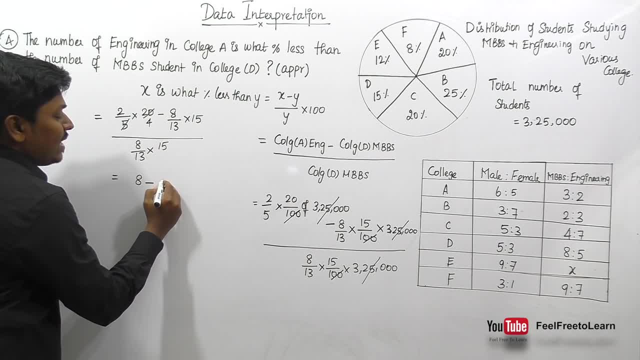 So 4 into 2 will be 8.. So 8 minus 8 into 15 will be 120 friends, 120 divided by 13.. Similarly, So 8 minus 8 into 15 divided by 120, divided by 13.. 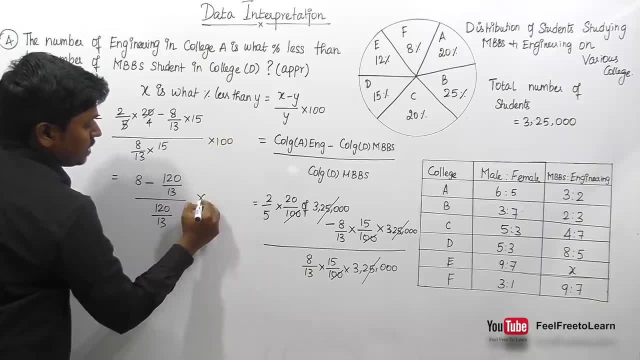 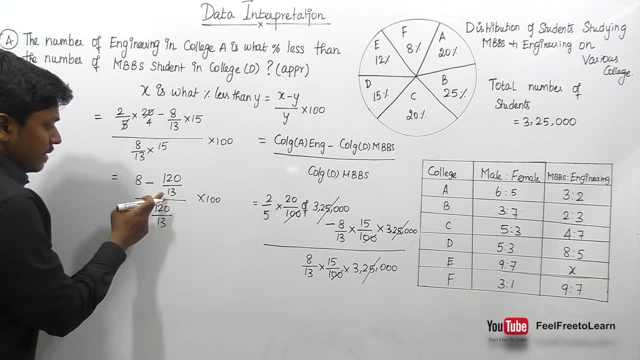 Friends, listen carefully- into 100, we missed, into 100, right. So into 100, into 100, similarly here to into 100.. Why? because x minus y, divided by y, into 100.. So, friends, I think we can take an LCM 13.. 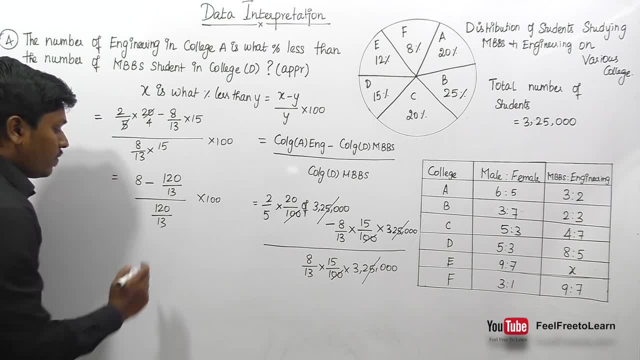 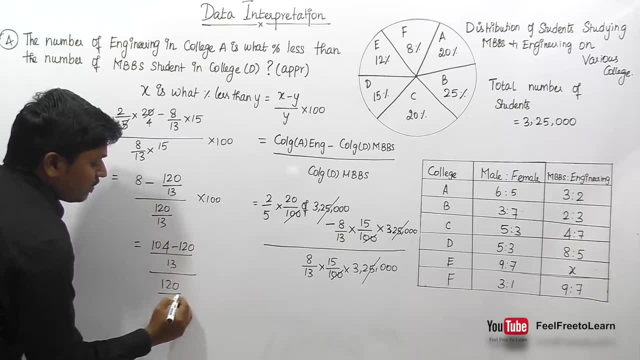 If I take LCM as 13,, 13 into 8 will be 104. So I can say that 104 minus 120 divided by 13.. Similarly, here it is 120 divided by 13 into 100.. So we can cancel this 13 and 13.. 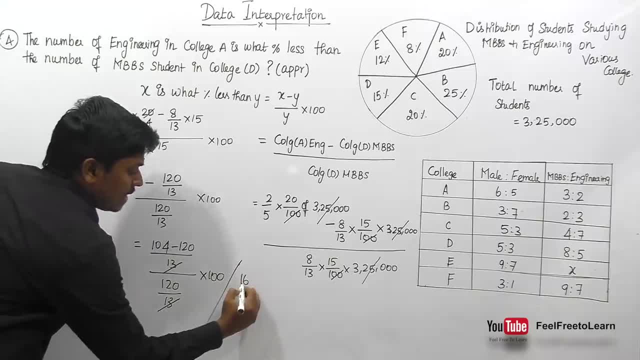 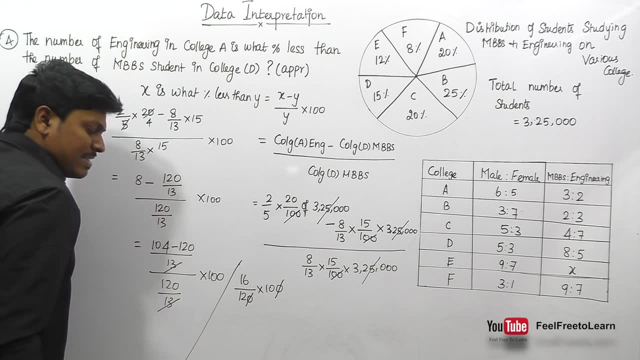 104 minus 120 will be 16.. So I can say that 16 divided by here values of 120 into 100. So we can cancel 0 and 0.. I think we can cancel this on 4 table.